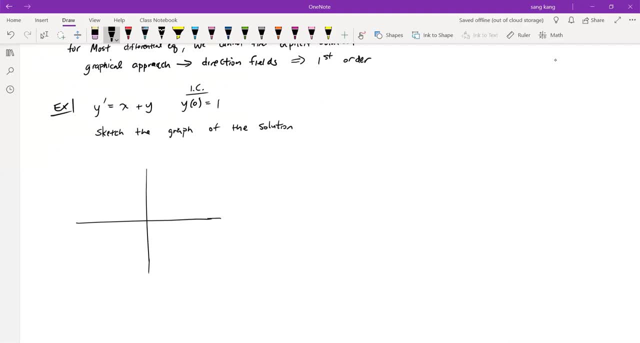 But essentially, what we want to do is graph. We want to graph all of the slopes pertaining to this differential equation. okay, So if this is my x coordinate and this is my y, I want to plot the tangent slopes, the tangents to my y, or just the slopes, in other words, the y prime values. 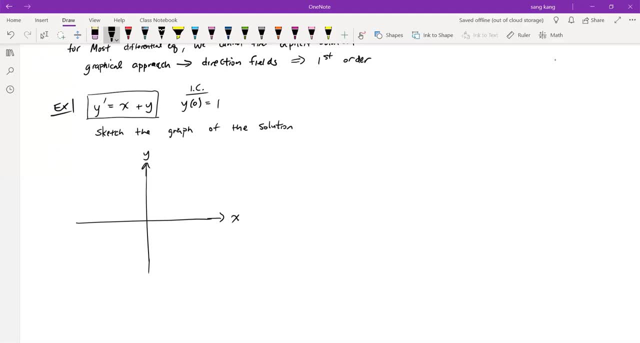 So essentially, I want to plug in values of x and y. I want to plug in values of x and y into this differential equation that I've boxed and basically draw. so to clarify, we can only use direction fields for first order. 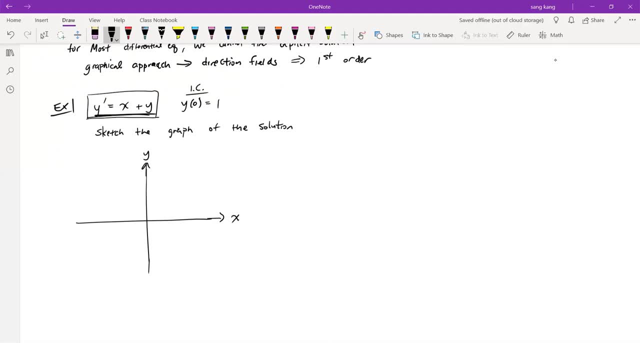 Yes, So this is for first order only. so with y prime values, okay, So all of these problems will only have y prime as the highest order. okay, So, as I've mentioned, we're going to plug in values of x and y into this differential. 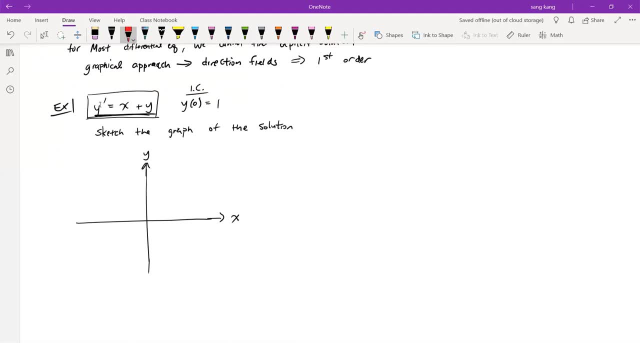 equation. We're going to plug in values of x and y into this differential equation and see what kind and basically draw out the line segments that's representing the slopes. So at 0, 0, x equals 0, y equals 0, we would have. so I'll draw this in red: the slope. 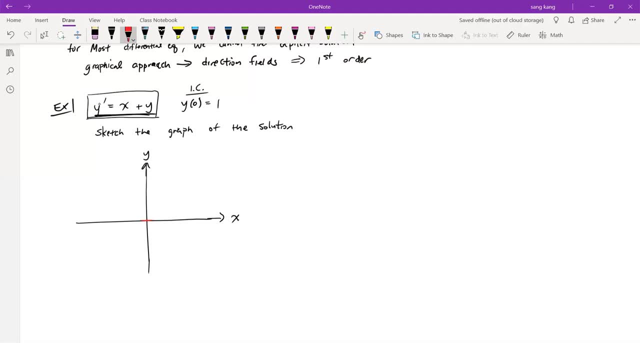 of 0. And then as we increase x values, so x equals 1,, x equals 2, 3, negative 1, negative 2, negative 3.. We'll look at it this way, Okay, So at at x equals 1, and y equals 0,, we'll have a slope of 1, actually, let me just draw. 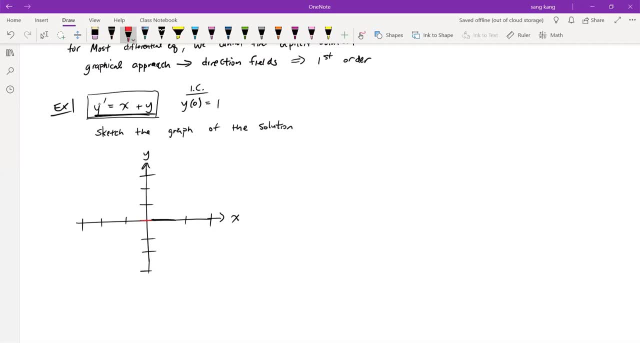 this. let me just write down the numerical value first. So 0, at this point we'll have 1, at x equals 2, y equals 0, we'll have a slope of 2, obviously we can see a pattern here, right. 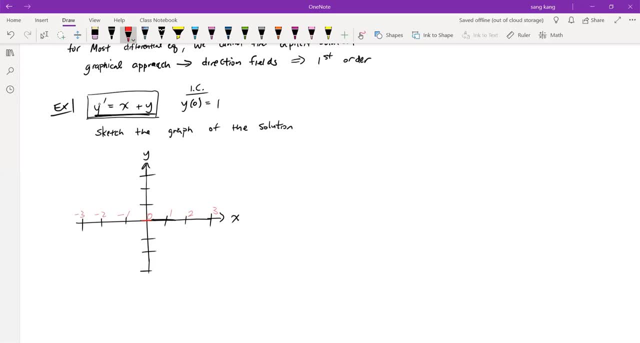 At y 1, x equals 2, y equals 0, we'll have a slope of 2.. Okay, At y 1, x equals 0, this will be a slope of 1.. At 1, 1, we'll have a slope of 2.. 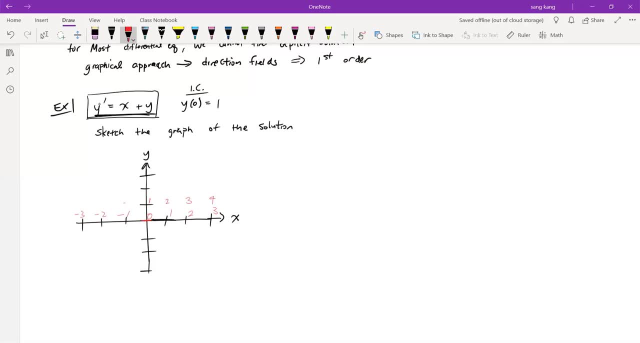 At 2, 1,, we'll have a slope of 3, and then you can see the pattern here. So this would be 0, negative, 1, negative, 2, so on and so forth. At x equals 0,, y equals 2,, this would be a slope of 2, 3, 4, 5, negative or 1, negative. 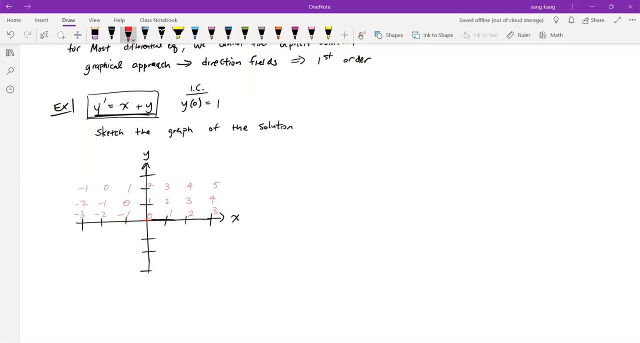 1, 1.. Okay, At x equals 0, negative 1, and we can do this for the rest of the graph. right, And I'll just do one more here, because this is really the only one that we'll need. 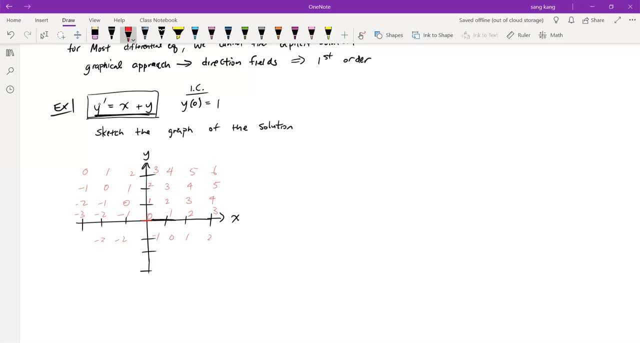 0, 1,, 2, negative, 2, negative, 3, negative, 4.. So again, if I was to draw approximately, Okay, Okay, Okay, Okay, Okay, I will put the tangent lines or the slopes for this. 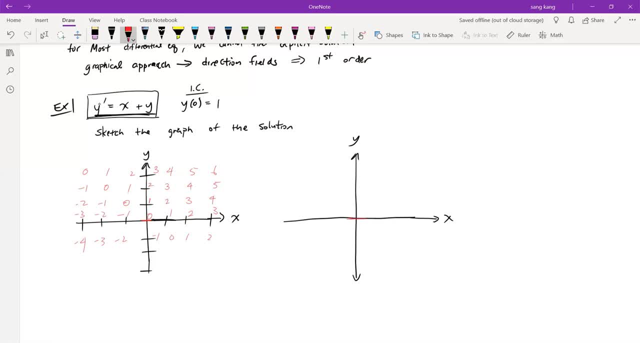 We would have a slope of 0 here. It looks like we'll have a slope of 1 here and then all Basically, all this, diagonals. here the slope will be 1,, right Here the slope will be 2,, so slightly steeper, and then, going along the diagonal, they'll 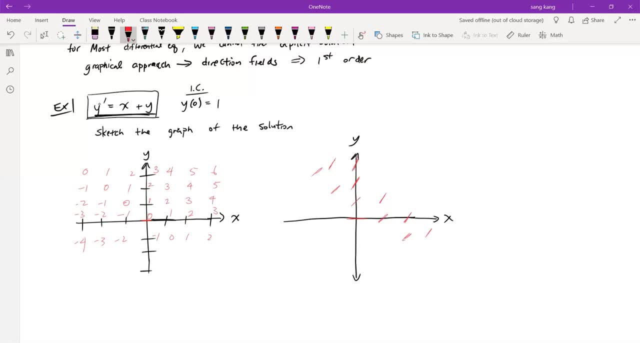 all be 2.. The slope will be 3 at this point, so a little bit steeper. and then going down at at a diagonal, you can see that they're also three, four, five, six. so four there, four there, if we go back this way. 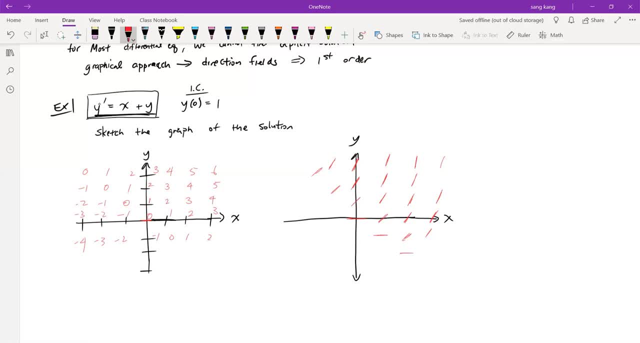 we have zero slope of zero going down this way right. slope of negative one, this way negative two, a little bit steeper, right, you get the point. so now we want to sketch the solution curve with the initial condition at y equals one, so zero, four, X, X, Y. 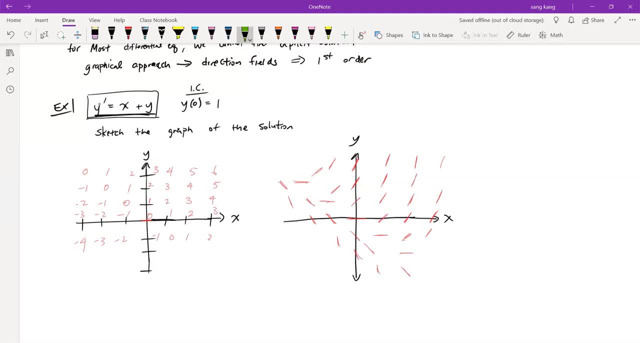 two to be zero and one. so we want to start with that point. so x equals zero, y one, and we want to basically trace. we want to trace all of these tangent lines. so it would go something like this: right at this point it would come back up and follow our solution curve. 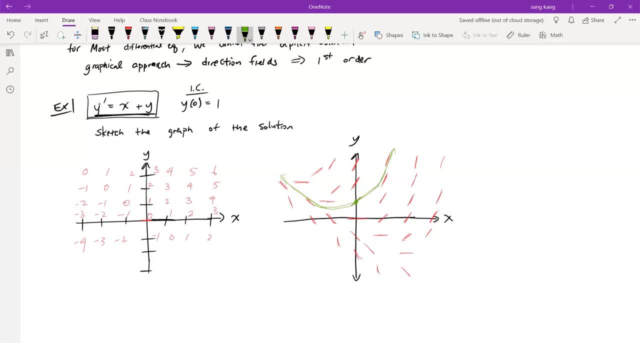 for this initial condition. so now we can use this solution curve to estimate um values of y on our curve based on this initial condition for this solution here. so at y uh for at x equals one. if we wanted to find the approximate solution for one, we would have maybe this point here, so this could be uh. 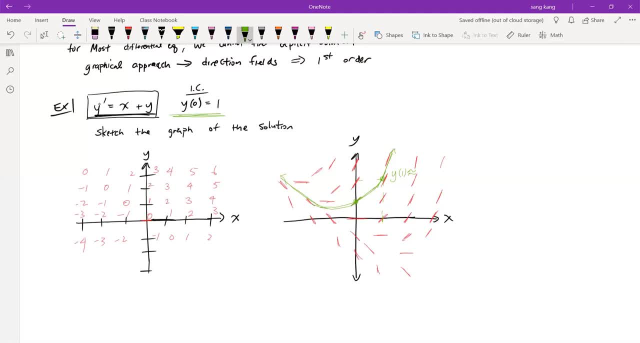 y one is approximately equal to two, and we can do this for other points. if maybe we look at negative three, so one two negative three, so at this point it would be this point. so maybe this is uh 1.6. so y at negative three is approximately 1.6. okay, so this is the graphical approach. 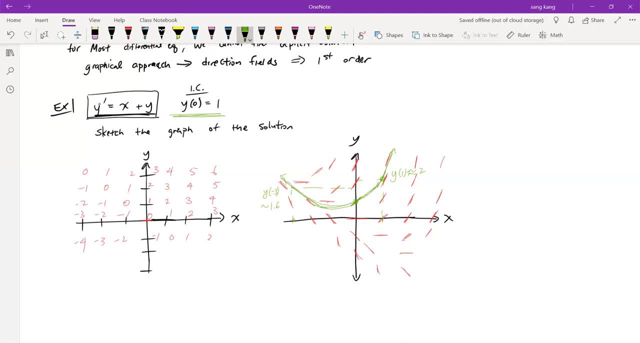 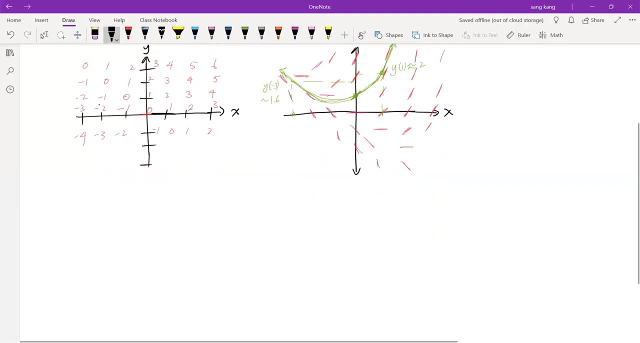 of coming up with the entire solution curve based on our given initial condition and then finding points on the curve using the solution curve that we just sketched. So any questions on that? so far, Okay. so in general, given y prime as a function of x and y, 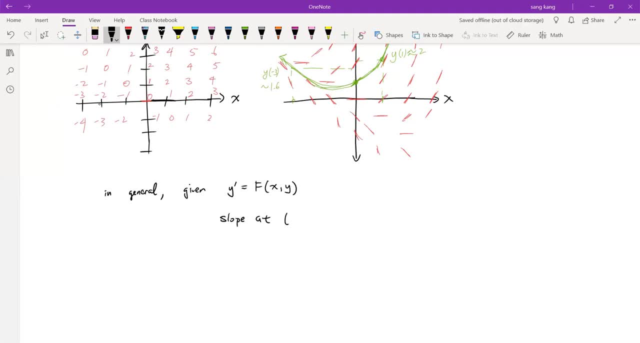 we can say: the slope at the coordinate x, y equals f of y right and all of the line segments showing slope. showing the slope is the direction field, okay, Or sometimes it's also known as a slope field, so that's a little bit more clear: direction or slope field. 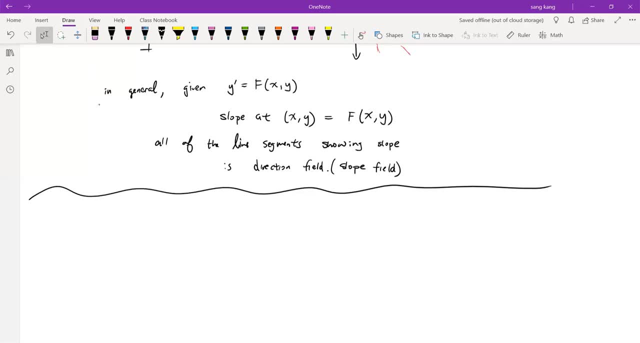 Now. so when we have a differential equation, we so we talked about this last discussion- when we have a diff eq of the form y, prime equals, let's say, g of y. remember these are. this doesn't have any x terms, so no x terms. right, we call this. 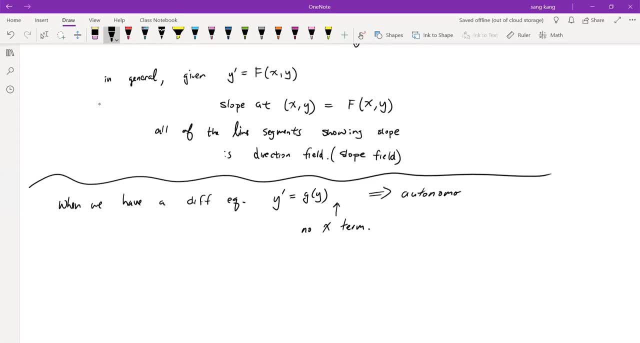 autonomous. these are called autonomous differential equations And remember there are a few implications from this. we said that y is going to be a constant and y prime is going to equal zero. So we did. I don't know if you guys remember we had a couple. 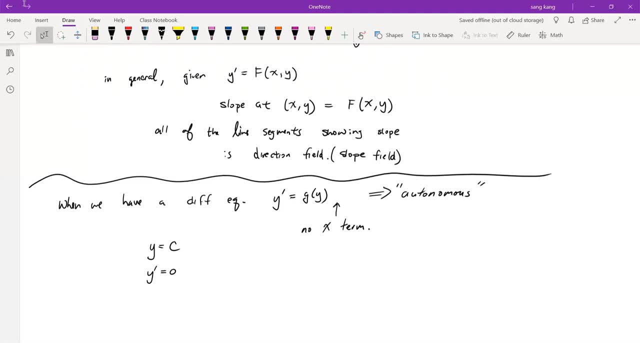 on the last worksheet I went through a handful of examples where this was the case And we set dy dt equal to zero and we solved for values where the slope was equal to zero and we called them equilibrium solutions, right? So you have to have your, your differential equation, is it needs to be? 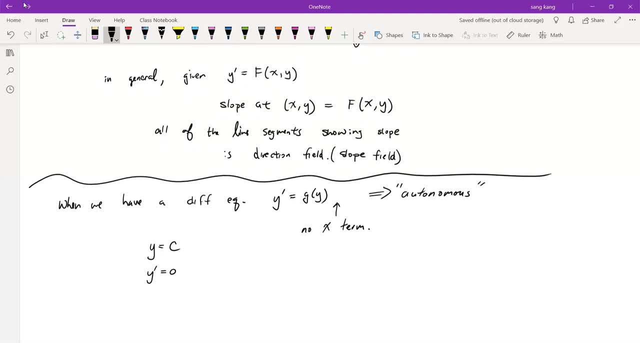 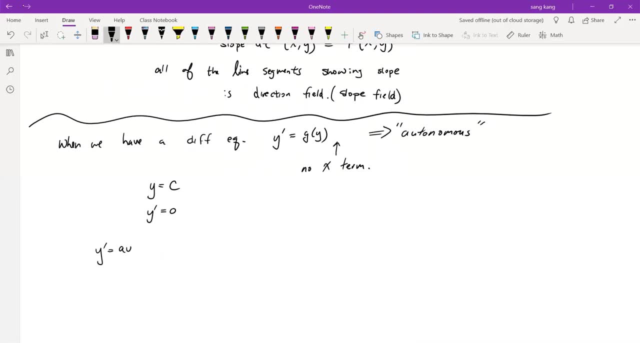 autonomous in order to have these equilibrium solutions. So let's look at one of the examples that we went over. So this was y prime equals zero. So let's look at one of the examples that we went over. so this was y prime equals a. y was one of the examples we looked at and, of course, if a does not equal zero, 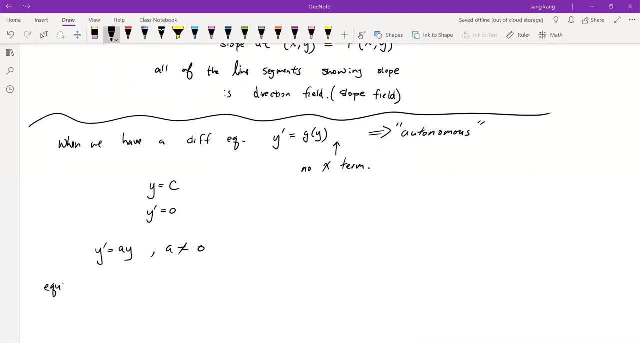 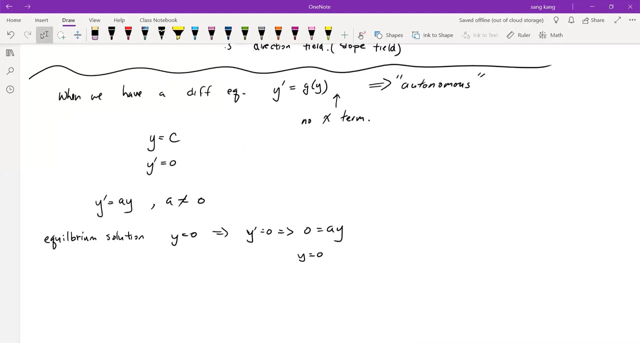 one of the equilibrium solutions for this. so if we're the only equilibrium solution would be: i equals zero right, and this comes from: if y prime is equal to zero, then zero equals a y. therefore y has to equal zero right, since a is not zero. now we want to talk about stable when we look at, when we look at equilibrium. 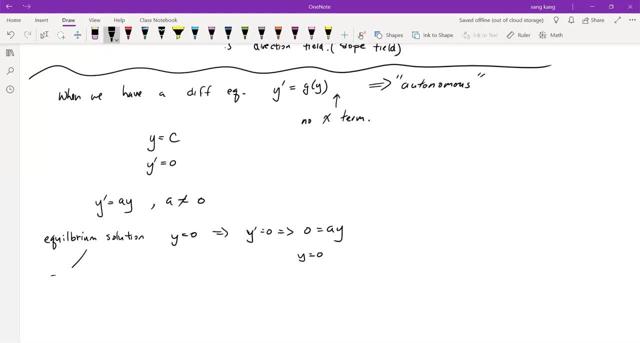 solutions. it could either be stable or unstable, and what does that mean? so if we plot y versus, or y prime versus y, so now note, this is not. this is not your slope field or direction field. you have y on the x-axis and y prime on the y-axis, right, what you're normally used to. 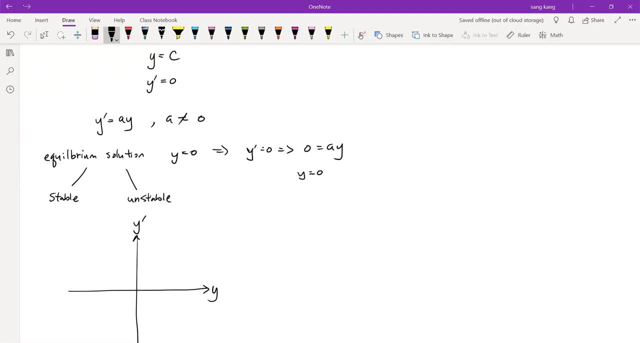 but um, instead of x and y we have y and y prime. so we're graphing the y coordinate with respect to the slope. so for this differential equation here, a y if a was positive, if a is greater than zero, it would just be a straight line going through. 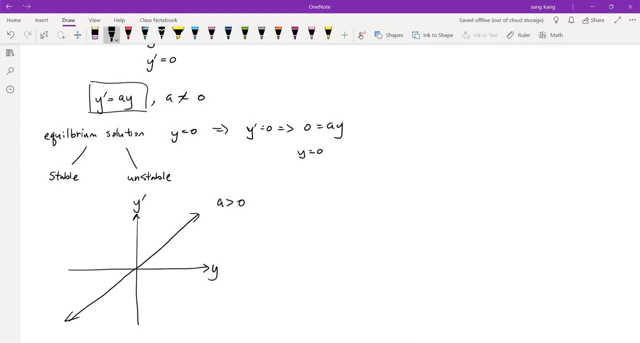 the origin right if a was greater than zero. if a is less than zero, then we would have this case right. so this is for a less than zero, and this is still y and y prime. well, the the y prime values here show us the slope, so our solution is going to be stable. 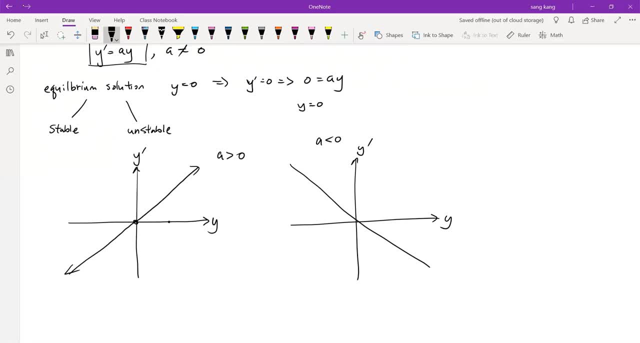 so when we pick, when we pick a value of y, we can pick a random value of y that's on either side of our equilibrium solution. is our equilibrium solution right? So this is when y prime is equal to zero. This is our only equilibrium solution for the differential equation that we're looking at. If we pick a point above it. 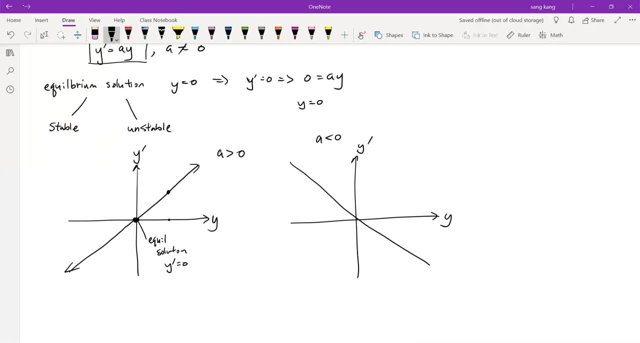 so a y greater than our equilibrium solution. and we look at the slope. we have a positive value here, right? So if your slope is positive, what is it going to do to your solution? It's going to increase the y values, right? So it's moving away from your equilibrium solution. 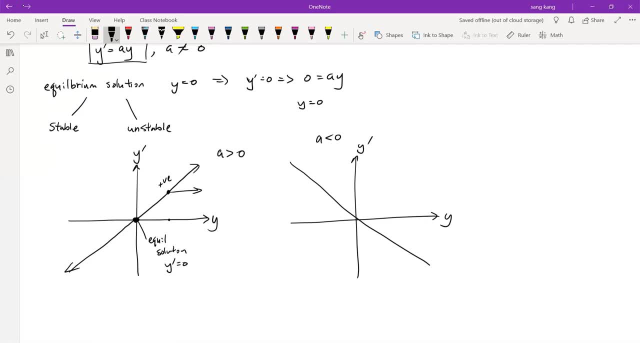 Now let's look at a point less than the equilibrium solution. so to the left of y prime, y equals zero. So that's, if we look at this point now, our y prime is negative. we have a negative value here, so that means our slope is negative. so how would that affect our solution curve? 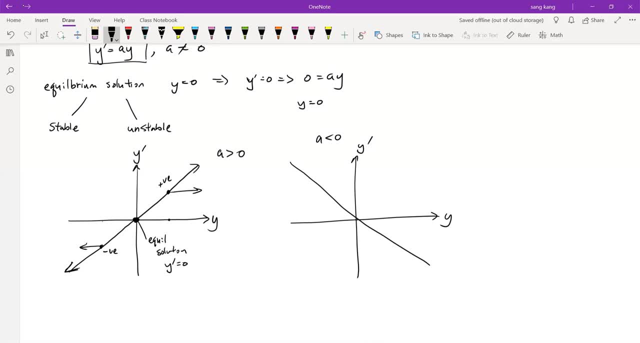 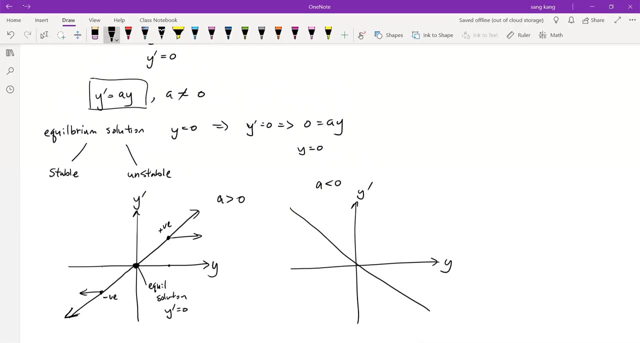 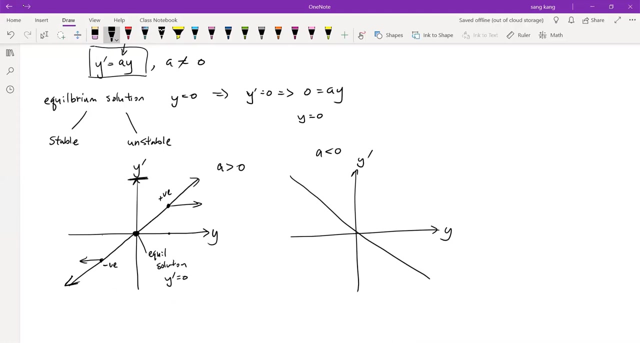 how would that affect our y value? it would subtract from it. so, basically, when you have an a or your slope, your slope of your differential equation- okay, not, i'm not talking about this y prime value, i'm talking about the slope of your differential equation. when that slope is positive, you're going to have an unstable solution. okay, and all this means is: 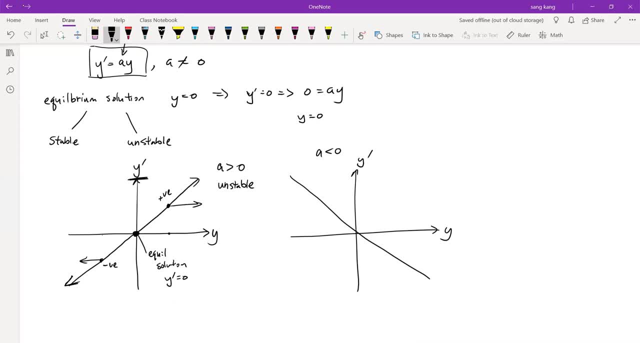 if you're not exactly on the equilibrium solution, that means it will deviate from the equilibrium solution. so think about this as a ball on a hill. if it's perfectly centered right on the hill, it'll stay there, but if you have any sort of deviation left or right, it'll roll off the hill. 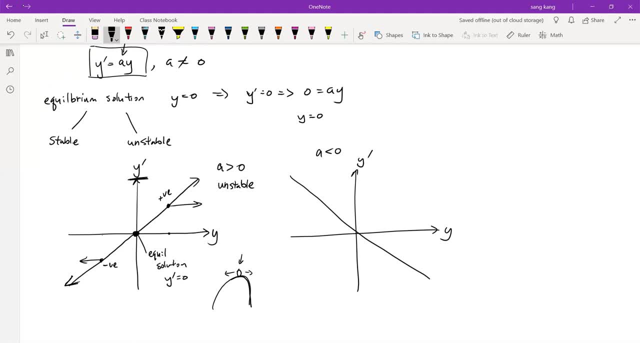 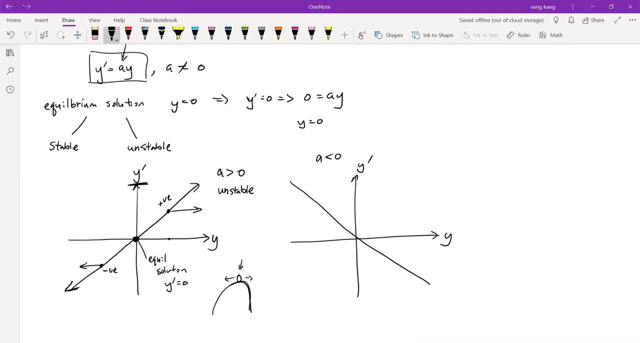 so that's kind of a good analogy that i've heard for explaining this. so now let's look at the case where a is less than zero. well, if a is less than zero, so basically the slope to your differential equation, and we still have this point here as our equilibrium solution. 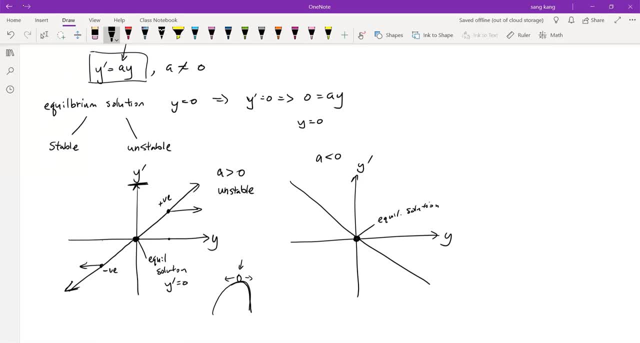 and we. if we look at two points, uh, one above the equilibrium solution and one below. so if we look at this point here now, our y prime is negative, right? so that means our y value is going to go towards this direction. right, we're going to subtract, we're going to subtract. 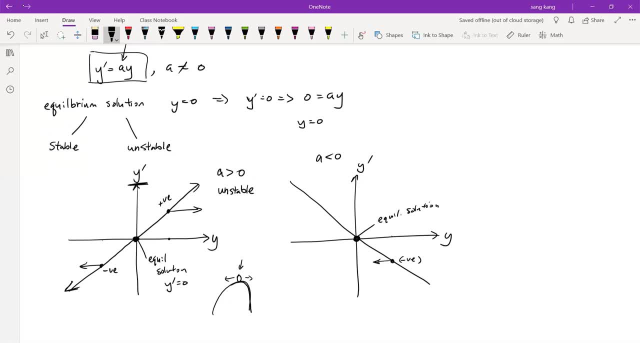 our. since our slope is negative in our, in our equation, we're going to, we're going to subtract from our overall y value, bringing us closer to our equilibrium solution. now, when we pick a point less than our equilibrium solution, we have a positive slope. so again that's going to add to our y values. so it's going to again bring us closer to our. 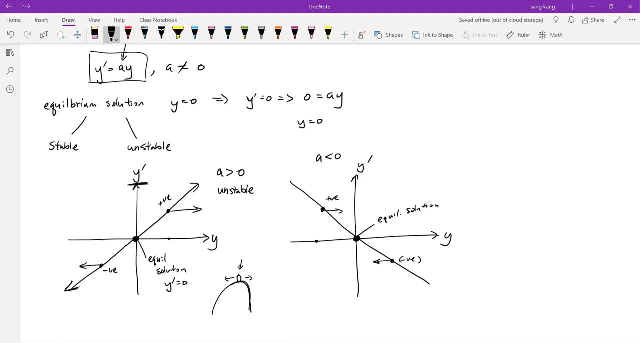 equilibrium solution and, as you can see, doesn't matter where you are on our curve here, it's going to bring us towards our equilibrium solution. so this is considered stable, okay. so so for a linear case, you if actually this is true for both linear and non-linear. but let's look at, we'll just look at. 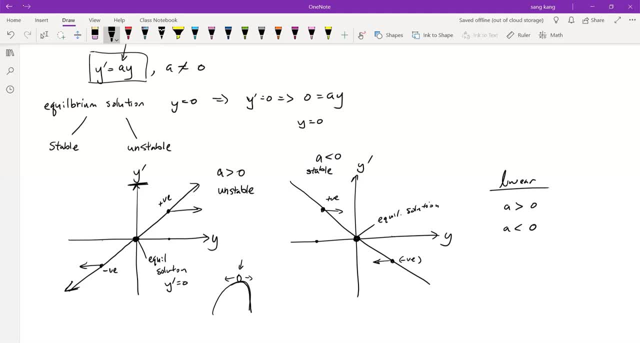 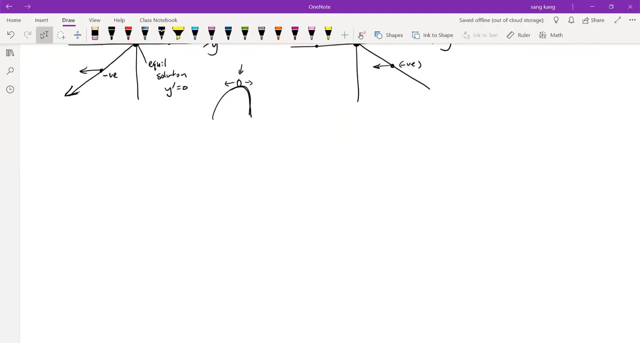 this first. so when a is greater than zero, we're unstable, and when a is less than zero, we'll have we'll have a stable condition. okay, so now what happens? so we also looked at another example where our setting y prime to zero, and then you'll see that our y is equal to plus or minus one. okay, so these are our equilibrium. 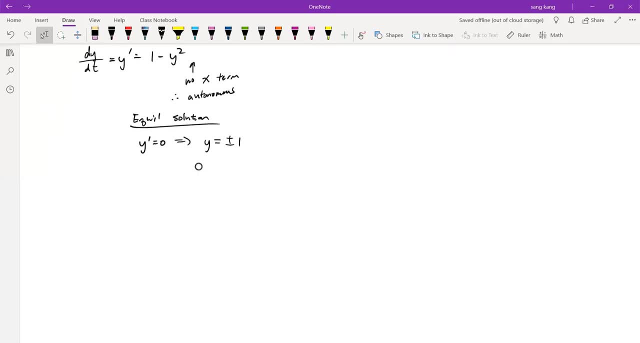 solutions. so now again, I'm not graphing. I'm not graphing the direction field right now. I'm graphing y, prime versus y, okay, so this will look like this, and then I'm going to go ahead and do a little bit of a probability test and the solution of this is going to look like: 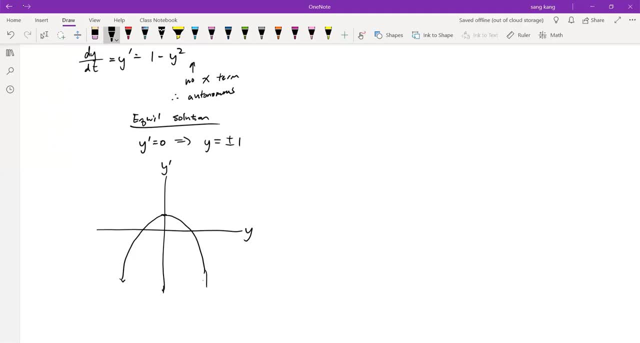 so we start at one and it opens downward right. so this is: this is y prime equals one minus y squared. and then, as you can see, these are our equilibrium solutions: 1 and negative 1. so y equals 1 and y equals negative one. so now we can kind of do the same thing. so all of these equilibrium solutions compare, and, dads, all of it is bigger than 1. so that was when we 왜� did this problem. okay, so, and we, yeah, we can kind of do the same thing. so all of this equilibrium, don't, all of theseenment for all of thesewohl solutiens, your homogenous 참 may be forward and remove yprime by doing something that should be done, right, but in general we find that here we 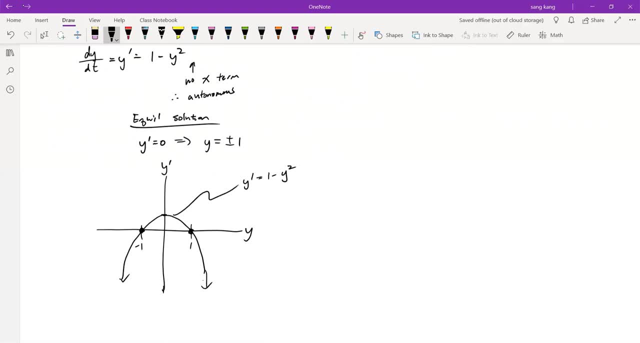 all of these equilibrium solutions, the stability of our equilibrium solutions, is a local behavior, so you're going to look above it and below it, okay, so it doesn't have to behave that way. for every point below, let's say this point, it just has to be on an interval directly below that point. so 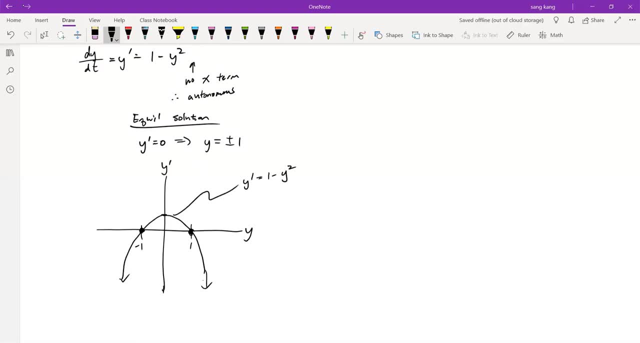 we can. we can check anywhere from negative one to one and see how the slopes, uh affect our y value. so if we pick this point here, so we're, we're looking, we're looking at this point here, we're trying to analyze the stability of y equals one and let's say we pick this point, our y prime is: 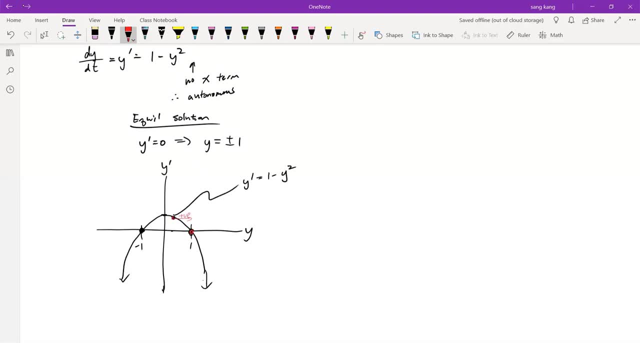 positive. so it's going to move us closer towards our equilibrium solution for y equals one. and if we pick a point above it, this is a negative y prime value, so it's going to bring again. it's going to bring us closer to our equilibrium solution at y equals one. 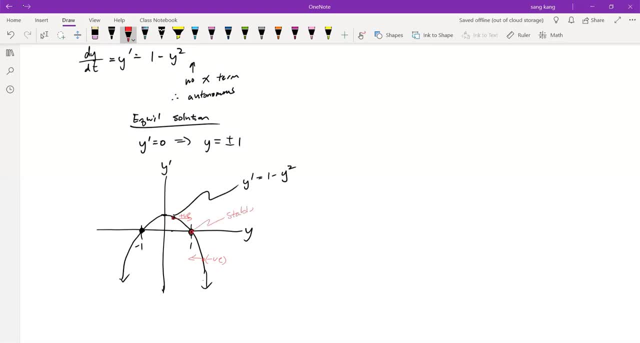 so, therefore, this guy here is stable, okay. so now let's do the same thing for this second point. for the second point: here we've already said that if we pick the point in this region, it's positive slope, so it's going to move to the right. 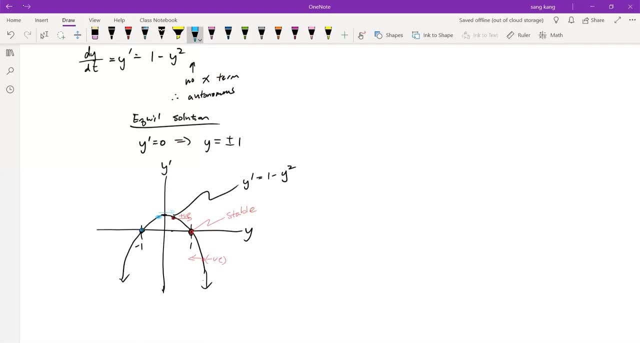 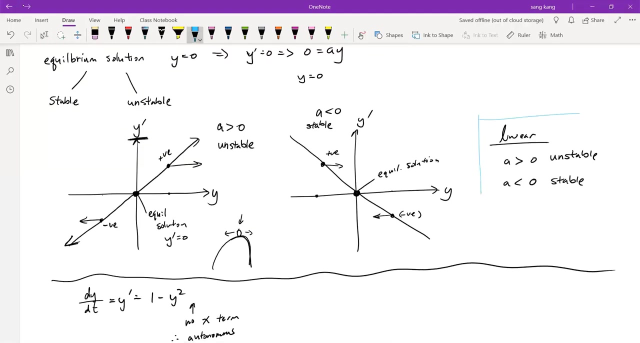 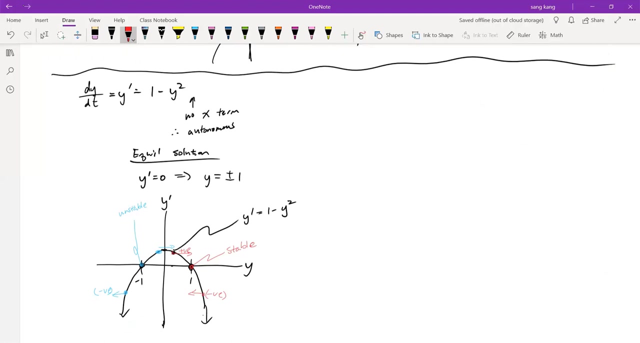 moving away from that equilibrium solution, and if we pick a point less than y equals negative one, it's a negative slope, so this will move this way. so this guy here is unstable, and now we're doing this graphically, but our same general idea here will work. so what i mean by that is: we look at, we look at the tangent to our uh, to our equilibrium. 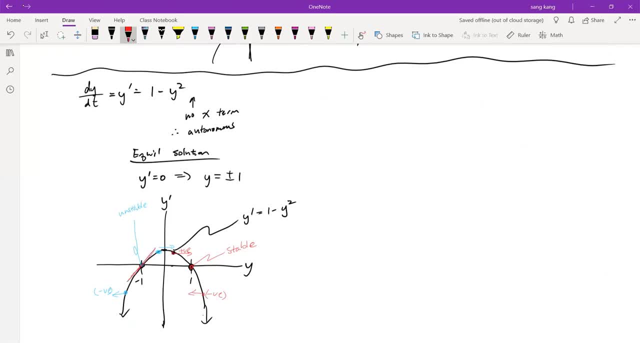 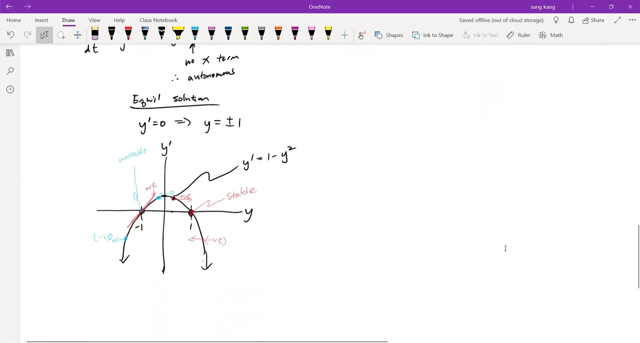 solution. so if we look at our tangent right here, that's a positive, positive slope, positive tangent, right? so what did we say before for the linear case? we said when a is greater than zero, it's unstable. well, it turns out in this tangent line is positive, it's unstable, right? so 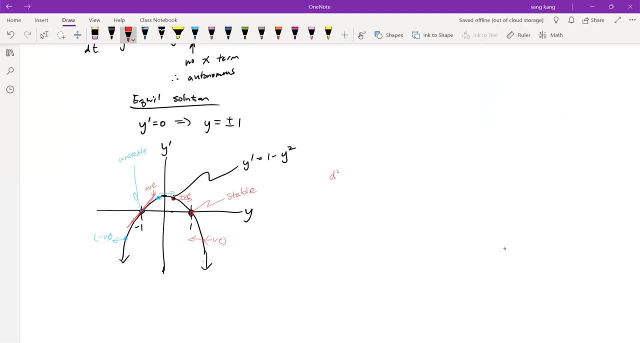 essentially this would be our second derivative right and evaluated at our equilibrium point right. so y. i'm going to denote that as y equilibrium. so this, this would be plus and minus one in our example here, And I put second derivative because of second derivative of y, because we're looking at the derivative. 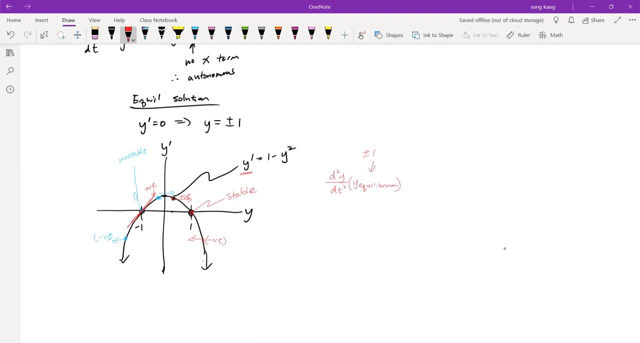 of our derivative equation, right? So that would be our second derivative. So if this value is greater than 0, we're unstable, And similarly, if this is less than 0, we're stable. And you can see that with this tangent line here. 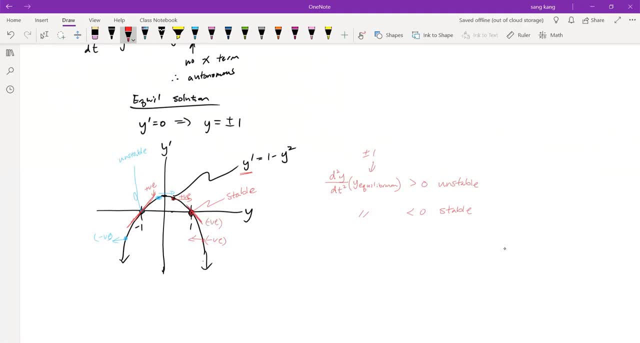 this is negative, And we've already shown graphically that that was stable. So this is how you could do it numerically, right. So any questions on that? I hope I didn't confuse anyone there, All right, So bear with me one second. 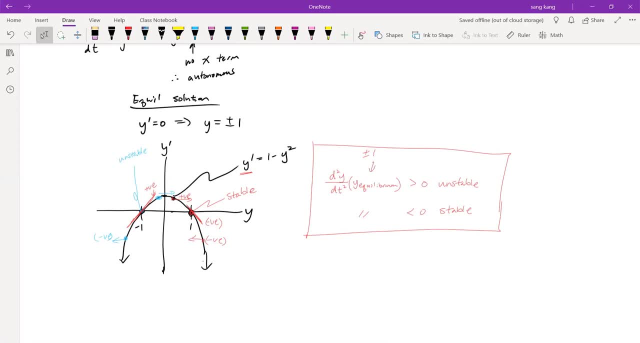 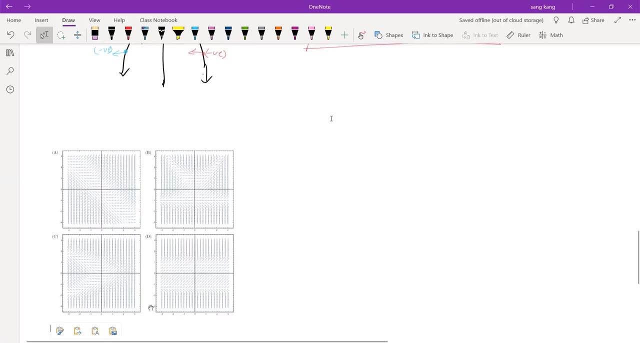 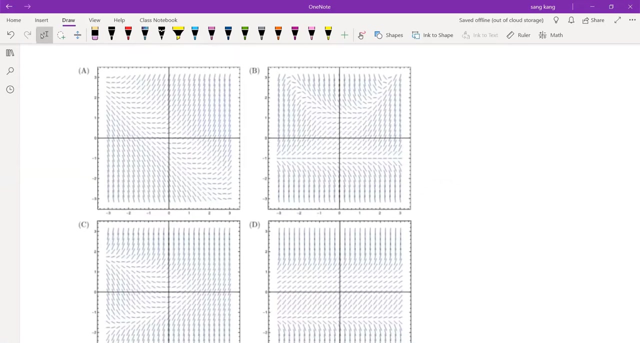 I'm going to do a screen clipping, So this is from the worksheet, But I'll paste what we need here, OK, So the first part of this problem asks us to draw some solution code on this direction. Actually, I'll just. 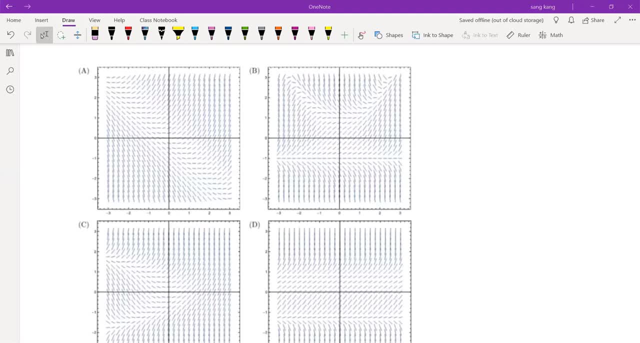 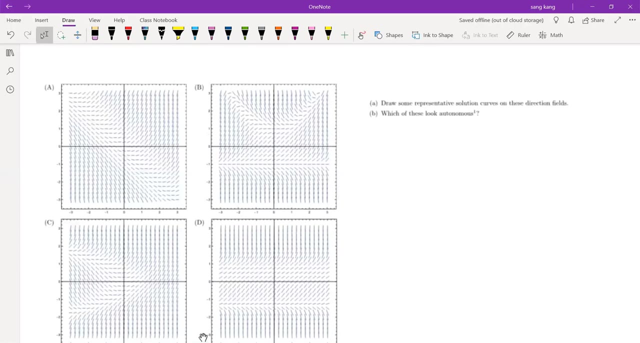 Here. let me OK. All right, Awesome representative solution curves on these directions. All that means is choose any initial value, doesn't matter, And we're gonna. We're gonna sketch a point here. So if we were to pick that point, all we're doing is connecting these tangent lines, or 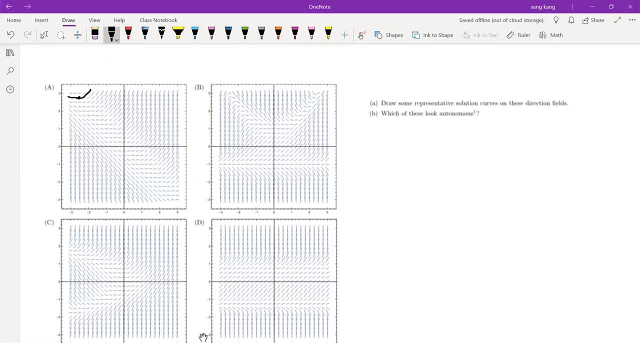 these slopes and our solution will look like that: We pick the point over here. you know it's pretty self explanatory. we're just following these tangent lines, right? So if we were actually on this, on this point here, this would be straight down like this: 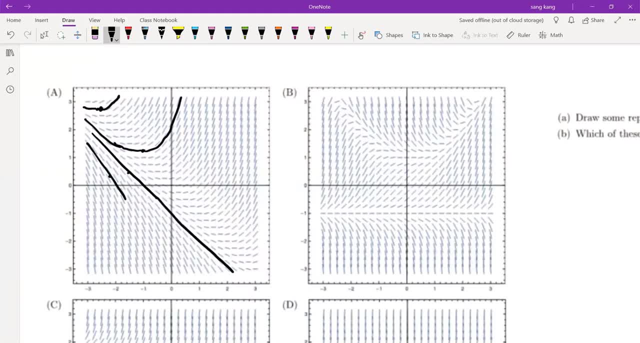 Right Looks something like this. That's too straight, Right? Something like that. I mean you can do this for all of these here. you can kind of see how these are behaving right. Come here. This, This, This. 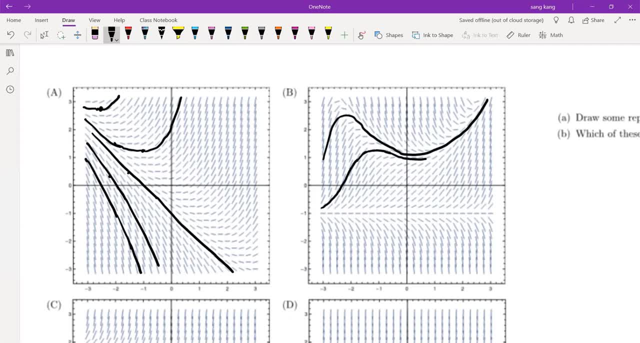 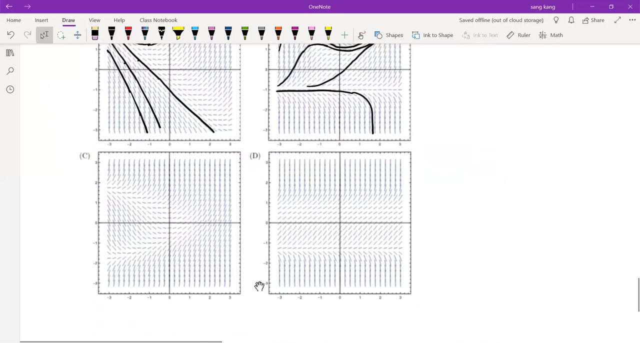 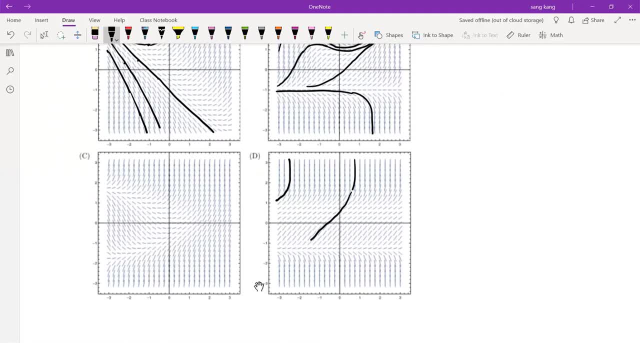 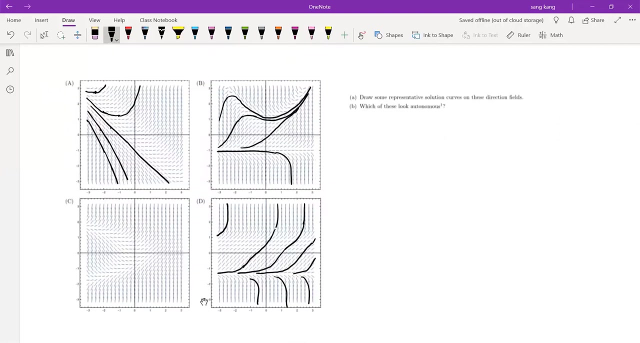 you pick, you draw some of these solutions curves out. our curves will look identical. However, they'll be shifted over, So this is actually a characteristic of an autonomous differential equation. Okay, Right, So now. oh, actually, I answered problem B. It's asking which one of these look autonomous. 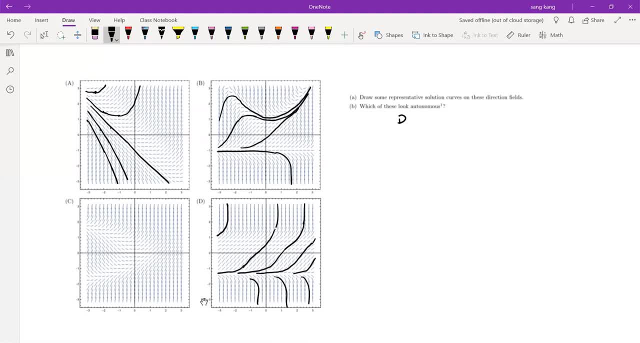 and it's going to be letter D here. And one one thing to note: when you have an autonomous, have an autonomous solution or autonomous differential equation. if you know for this, if you know one solution curve, you can find. 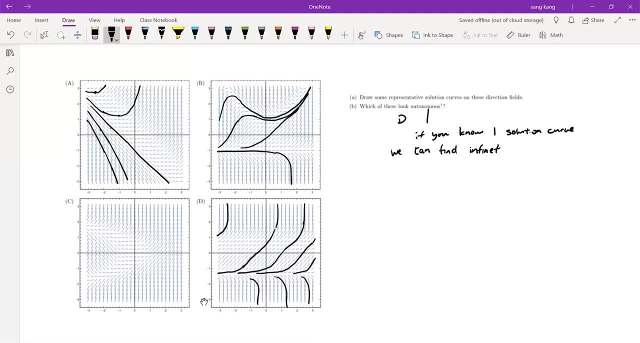 infinitely many solutions by shifting left or right. Okay, So this is one of one property of an autonomous differential equation. Secondly, slopes on a constant Y are equal. Okay, So this is one way of identifying the dyした Perfect. So you might think, well, A could be autonomous, But it doesn't. it doesn't fit this property. 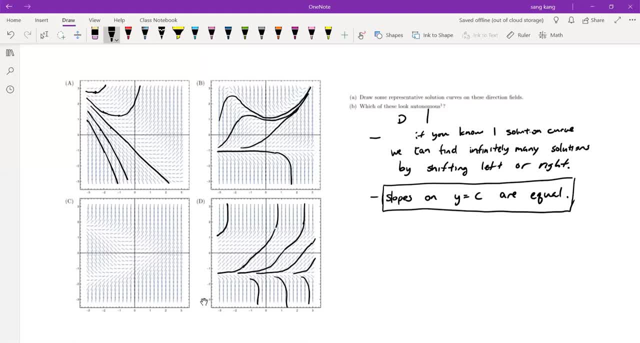 here Right. Or, or you might think, B is autonomous because we have- we have an equilibrium solution here, Right, But slopes on a constant Y. being equal is one of the properties that Right. So being equal is one of the properties of an autonomous equation, which means that 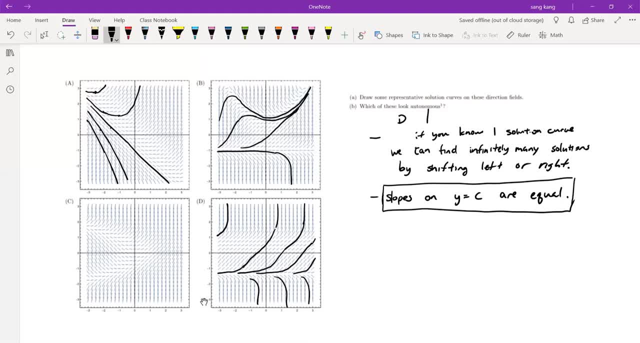 no matter where you pick your initial condition, you're gonna essentially sketch the same, the same solution: curve right and they're gonna look exactly alike. right, and all they're doing is shifting over a horizontal. horizontal and if you notice, let's look at all of these slopes. here's all of these tangent. 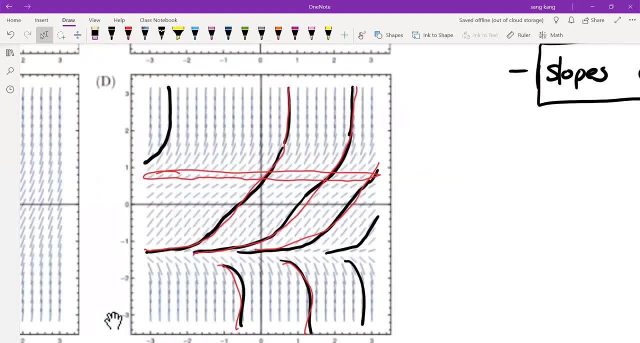 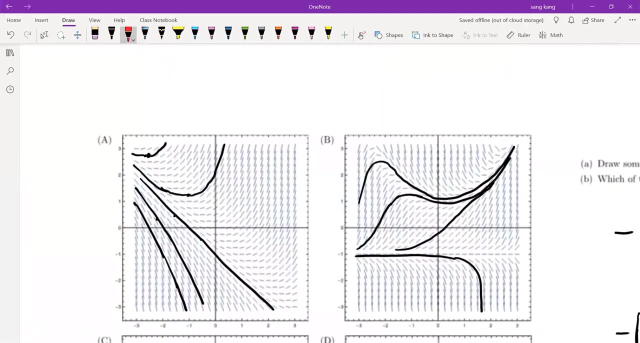 lines. right here we zoom in, they're the same along a constant y-value, right you know? for for any of these y-values they're the same, and that's not true for the other cases. the slopes change, and the slopes change for a constant line. okay, so that's one of the characteristics to be able to identify. 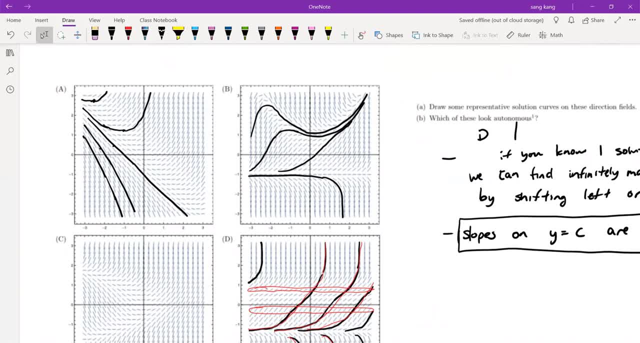 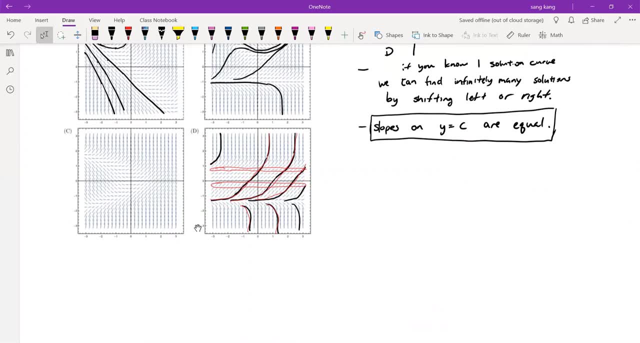 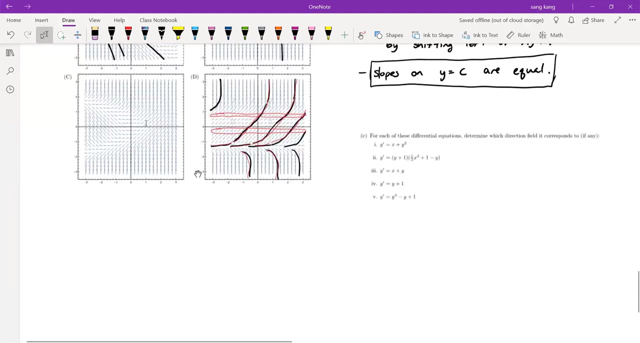 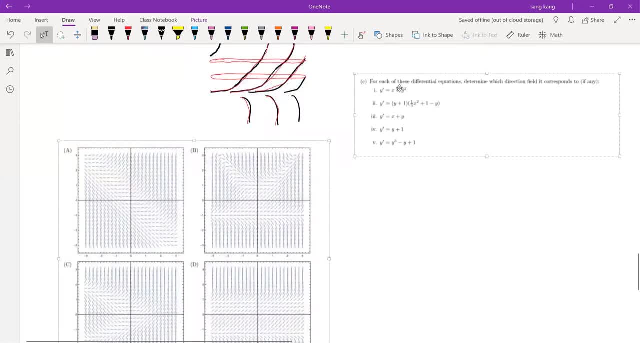 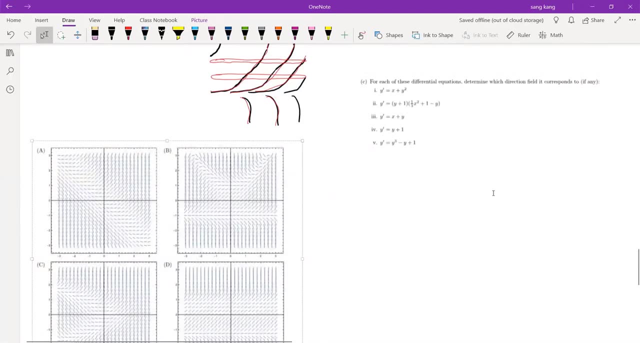 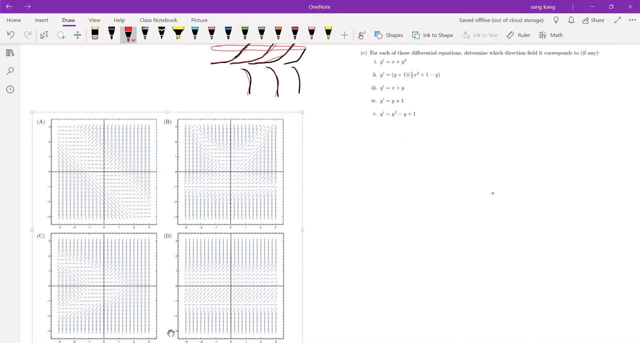 di the LEO. once this, the, the, the ever a types of questions where you have to match uh, I will say: I mean, obviously there's five equations, four of them will match uh, A, B, C and D, And one is just the random that was thrown. 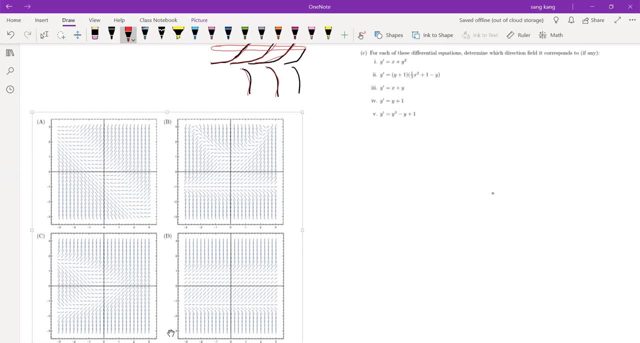 in there. Um, you could go completely brute force and basically look at plugin values for X and Y and, uh, find the slope and try to match it that way. And uh, you're going to have to do it for a couple of points just to get a few pieces of information. but we can use what we just 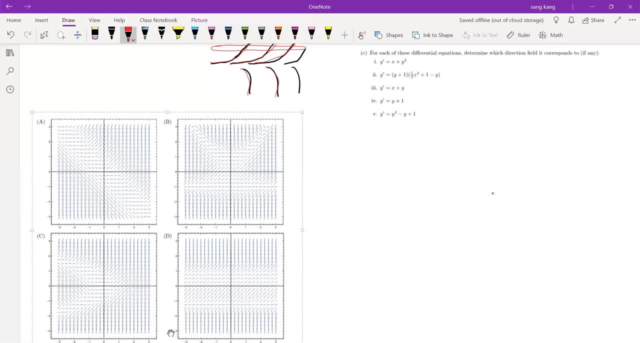 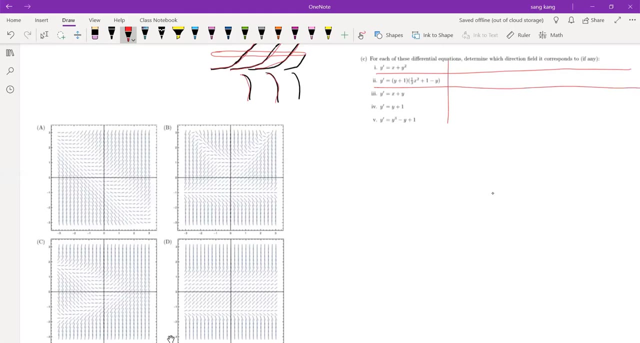 learned, uh, with the definition of autonomous, uh, to see if we can narrow down some of the choices. So let's look at this first one. So if we draw a table like this, so let's, let's check If, if any of these are autonomous. 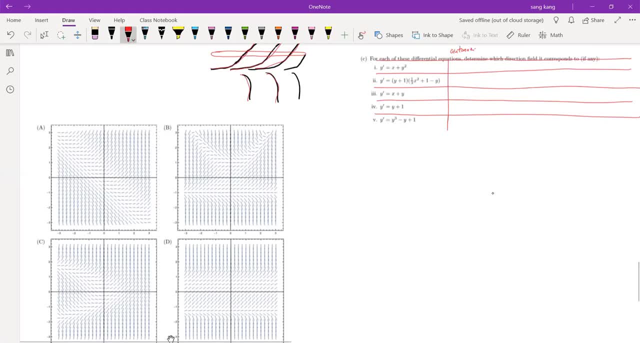 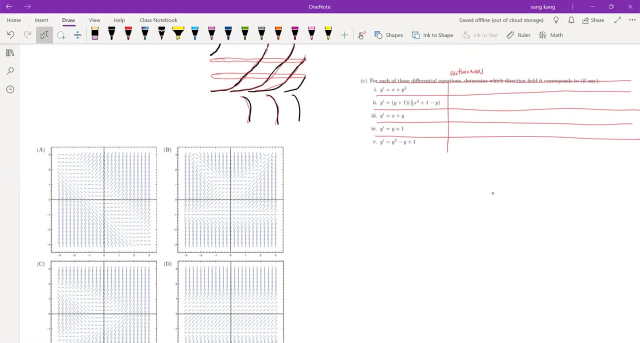 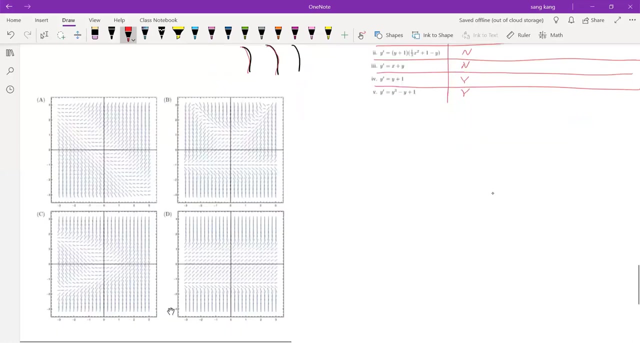 uh, is the first one autonomous? No, because we have X there. No, The second one also is a no. Third one has X's in it. So no, but these last two are yes. So we've already narrowed down four and five to D. Okay. 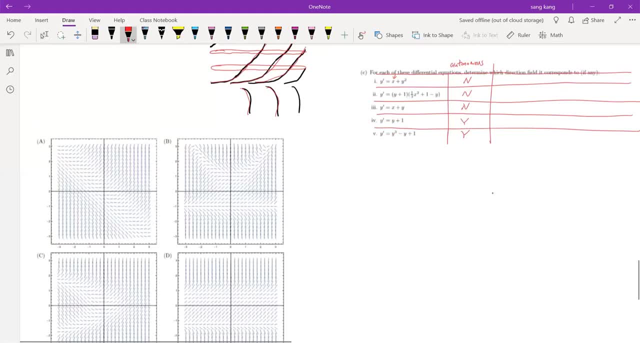 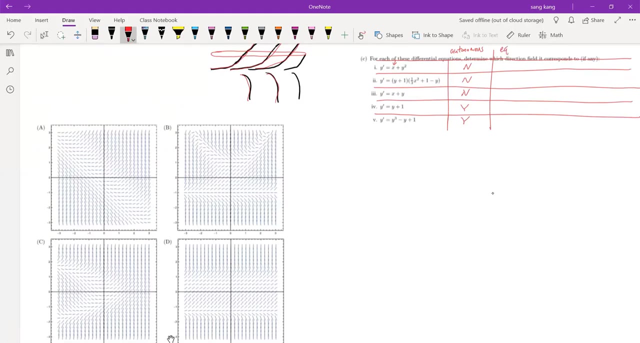 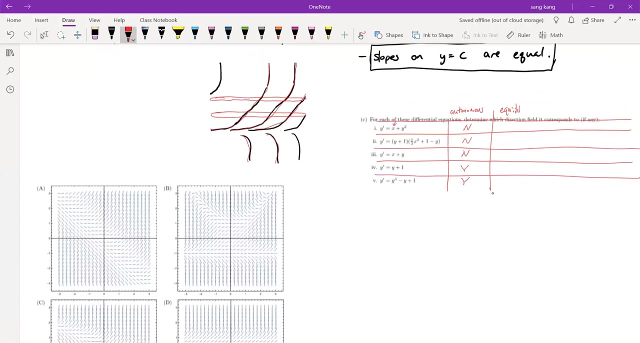 Uh, let's see, Four and five are D. Okay, So now let's look at potential equilibrium solutions. So, equilibrium, Equilibrium- Okay, Pen's acting up Equilibrium solutions, Okay, So the first one is not going to have any equilibrium solutions. 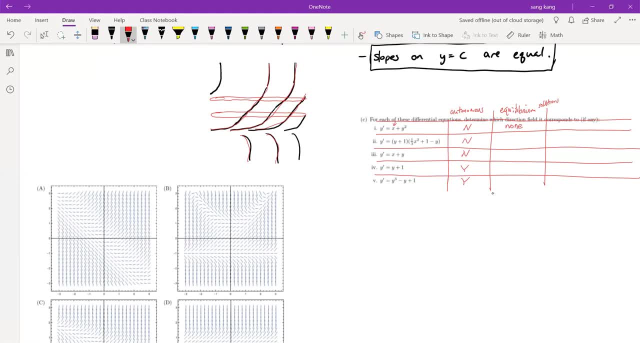 Um. the second one will have equilibrium solutions. even though there's an X here, Remember it's- equilibrium solutions are dictated by one. So equilibrium solutions are dictated by one y prime equaling zero, right? so this first term here, y plus one, this, that first term, if y equals negative one, we could have an. 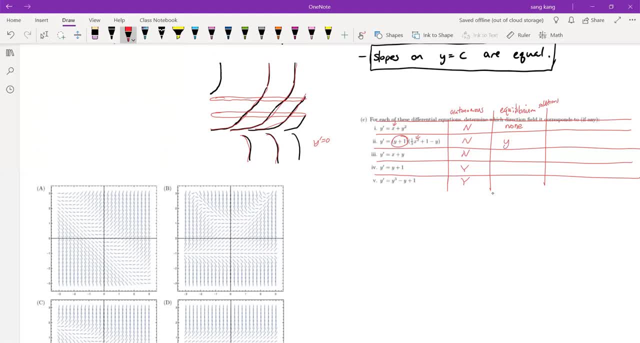 equilibrium case. this could be y equals negative one. and then, of course, the autonomous equations will definitely have equilibrium solutions. the first, so this. this third one is none, since, uh, it's very, it varies on x right um. the fourth one, again same as the second case: y equals. 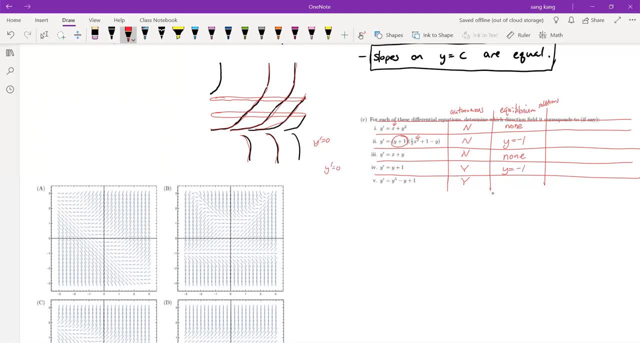 negative one. if we set y prime equals zero, you can get y equals negative one to give us zero. and case five: um, this is going to give us something less than a y, something less than less than one. okay, i, i haven't punched it in the calculator. 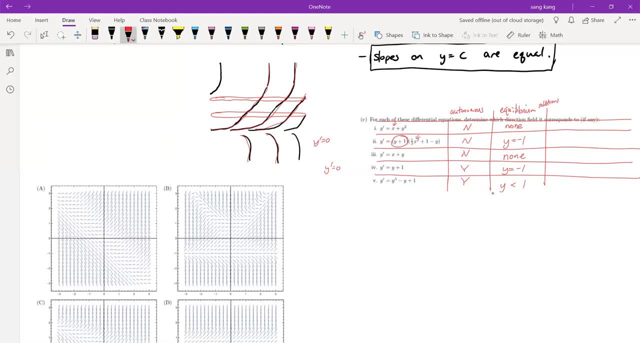 but it's going to give us something less than one, uh, and the graph of that looks something like something less than negative answer. it's going to look something like this and there's negative one, so we're going to get this point here, okay, so, based on this information, 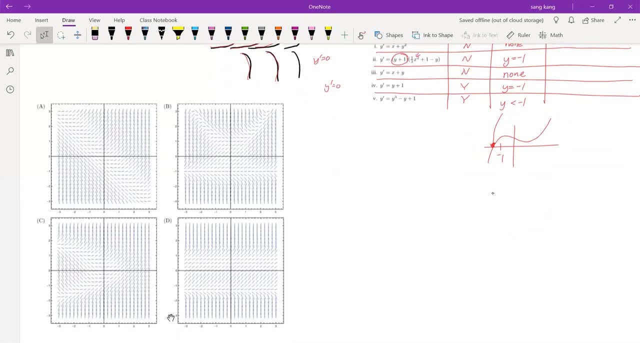 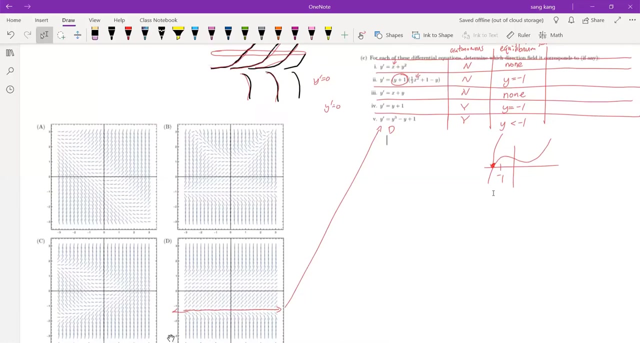 we should be able to dictate which one is d, right. so this guy has the equilibrium condition somewhere less than negative one, so we can say that this one corresponds to d and we can eliminate case four, because none other are autonomous, and this is obviously an autonomous condition. so 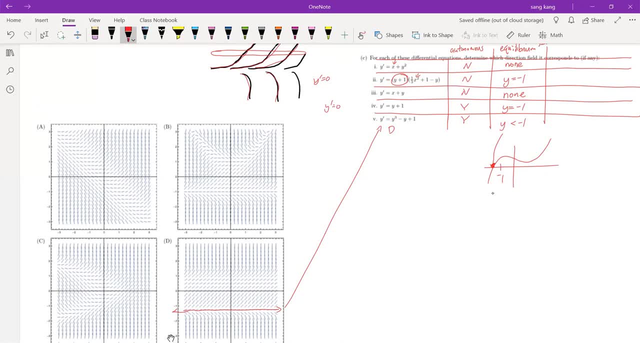 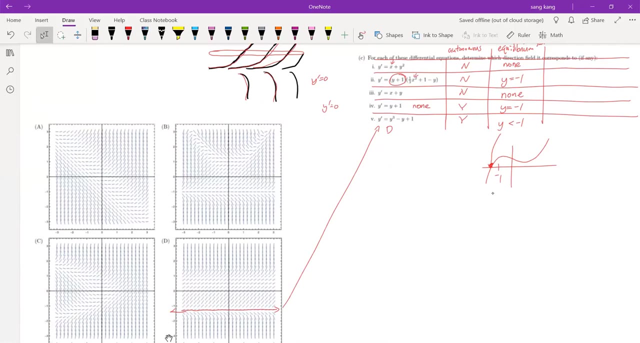 this is none, so this will not coincide with any any other uh solution curve. so now we have case one, two and three to match with a, b and c. we have an equilibrium condition here for case number two and as you can see here that's at negative one, so that it should correspond with this guy. that's the. 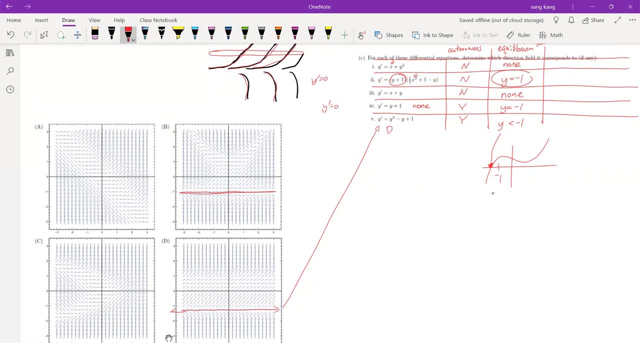 only one, so we can narrow it down to this guy here. so case two is going to be b, right, so we use that. b and d. so now, what about a and c? well, so this is what what i mean by the brute force method: we can plug in values we can look at. 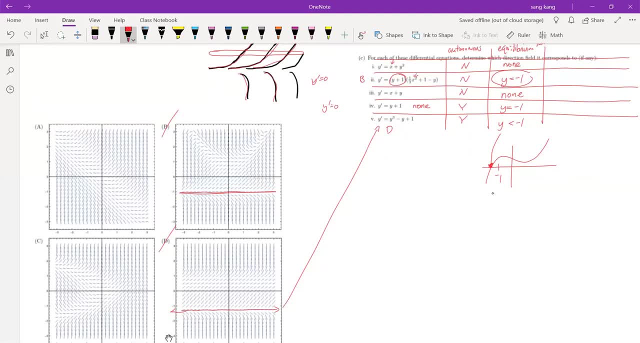 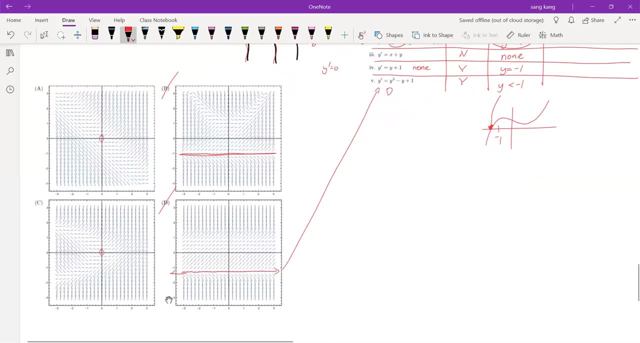 specific x and y coordinates and see which one it matches up with. so an obvious choice. so if we chose x, y at zero, this wouldn't really yield any results, any new information, because the slope at both of those points is the same, it's zero. so we should pick something that's. 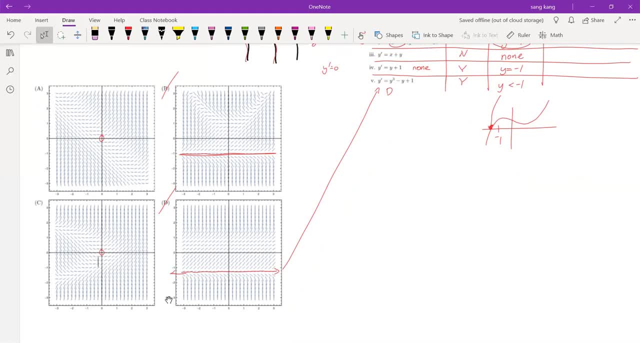 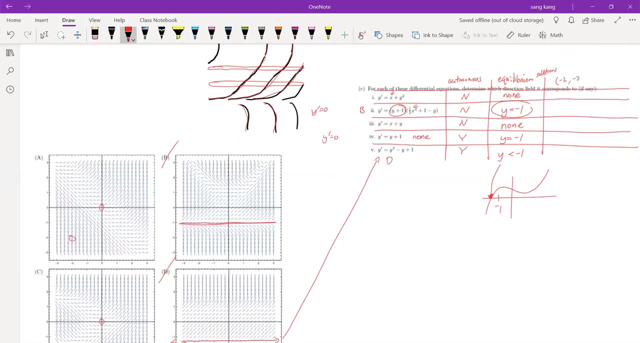 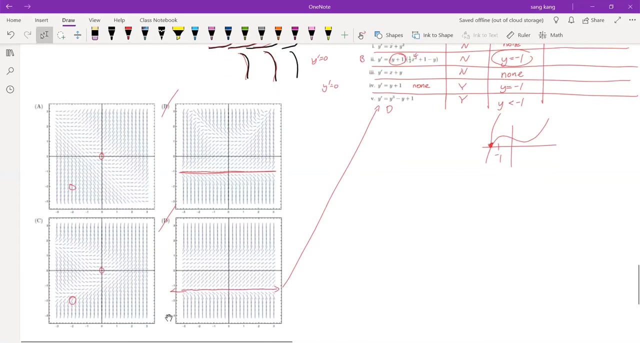 obviously different. so maybe somewhere down: negative two, negative two. so the slope here is negative, but the slope here is positive. right, so if we plugged in negative two, negative two, obviously the. if it yields a positive slope, we're going to have k c, so this is positive. 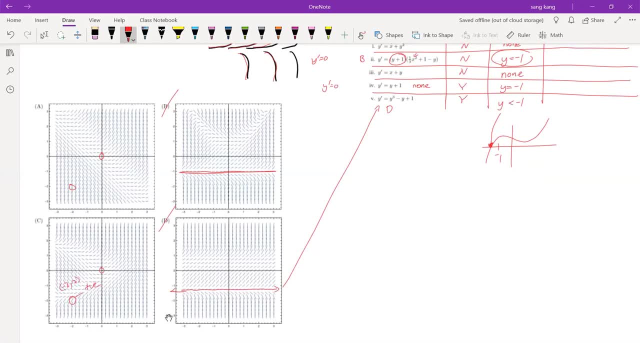 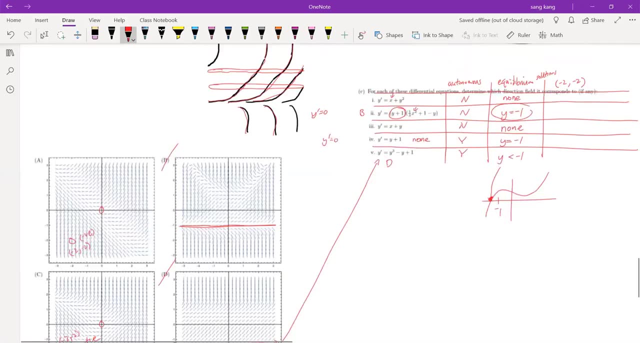 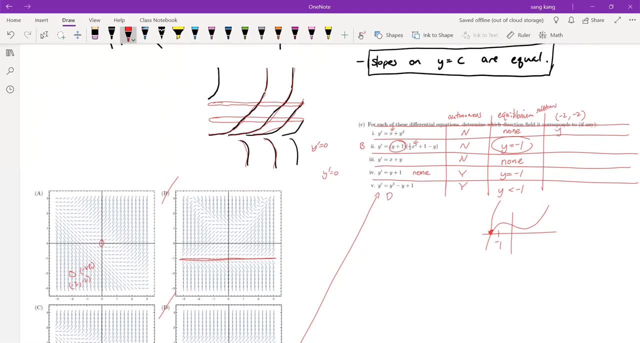 and this is for negative two, two, or sorry, negative two, negative two, and then this is negative, right, so we can use that as well. so if we plugged in negative two, negative two for this guy, we'll have y prime equals two, and this will be greater than. 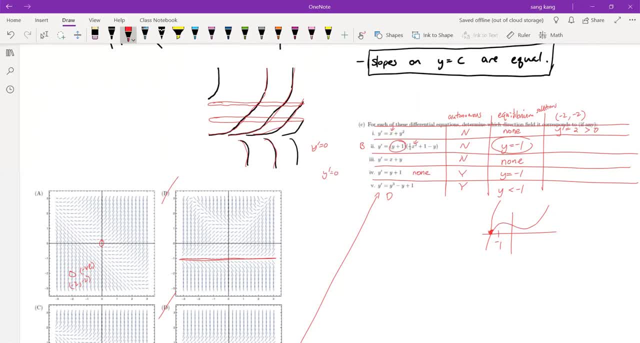 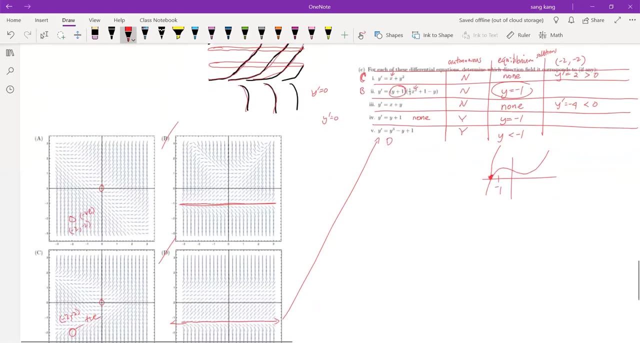 zero. so that's our positive slope. and then, just for good measure, let's check uh, case c: negative two, negative two. y prime would be negative four, which is obviously less than zero. so then our case one is the positive case. so that's c, and then case three will be matched with uh. 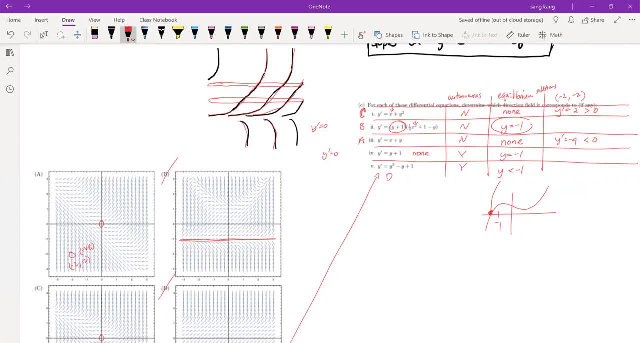 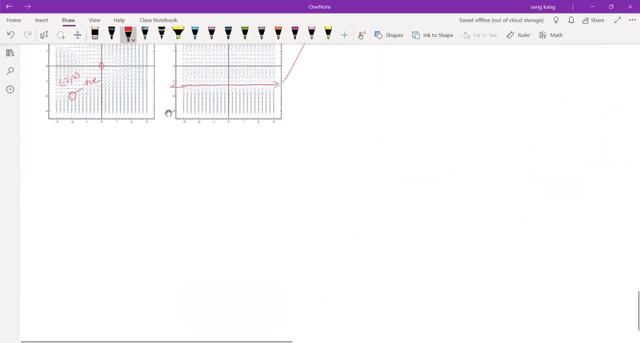 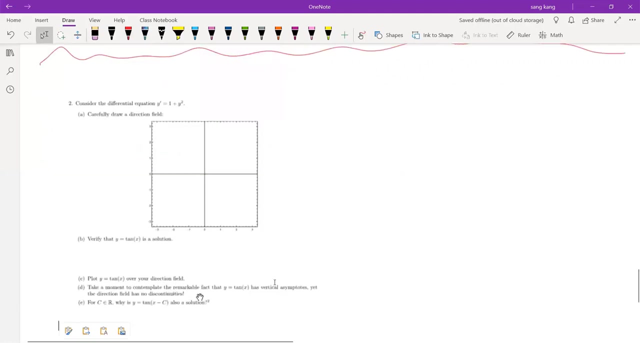 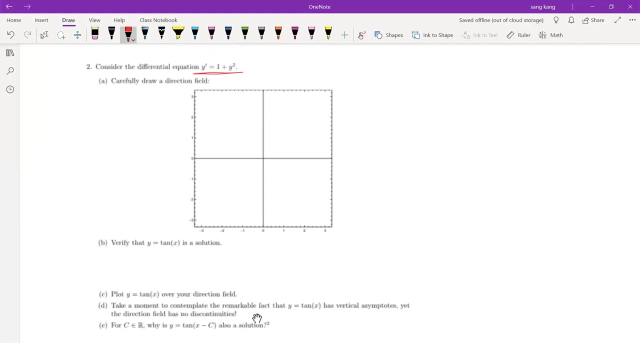 graph a: okay, any questions on that one? okay, moving on. all right, let's put this into the. okay, now we have this: differential equations. i hope you guys can see. uh, y prime equals one plus y squared. and now it's asking us to draw the direction. okay, so it seems like this is: 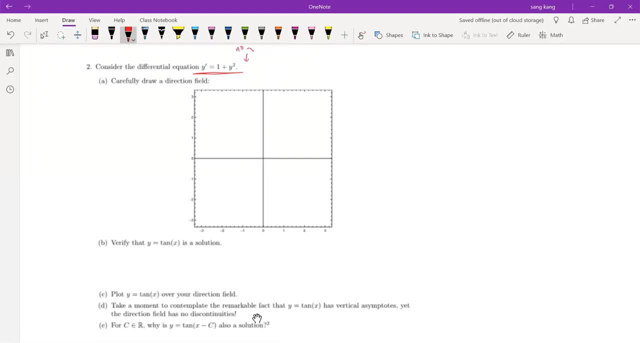 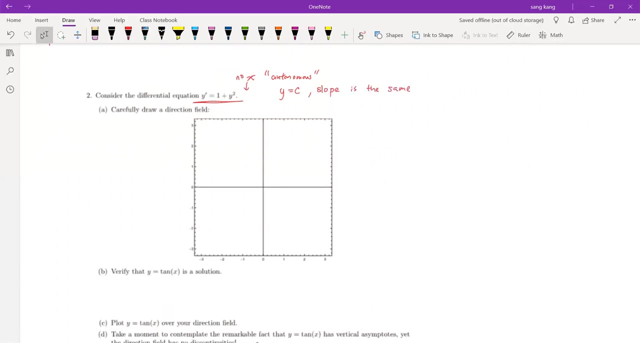 independent with respect to the negative suffix same. so that means that y equals 0, we're gonna have a slope of 1. right. at y equals 1, we'll have a slope of 2, so a little bit steeper. they kind of look the same. at y equals 3, it'll be even more steep, right, because it'll be 3 squared. 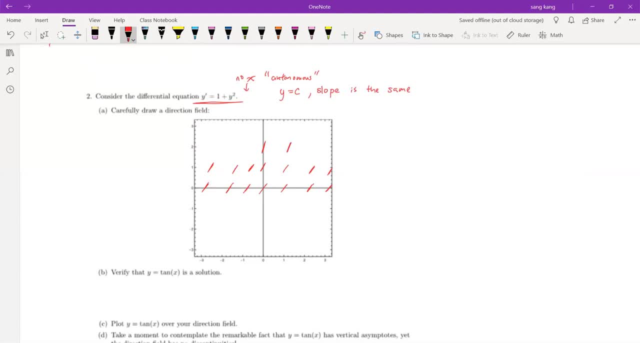 so the slope will be 10. so I need to be exaggerating this here. and at y equals- oops, I skip, let's skip. y equals 1. oh, you get the point. so 3, this will be even more steep. I think I skip the number. and then for y equals negative 1. 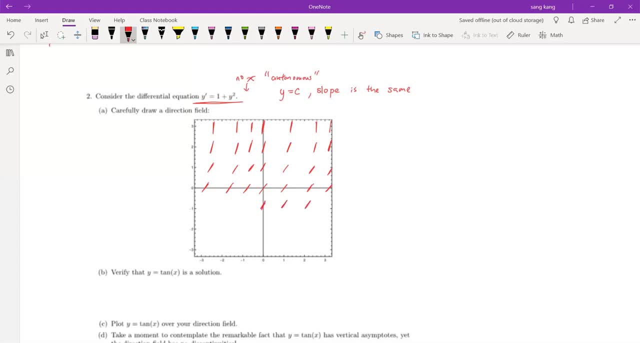 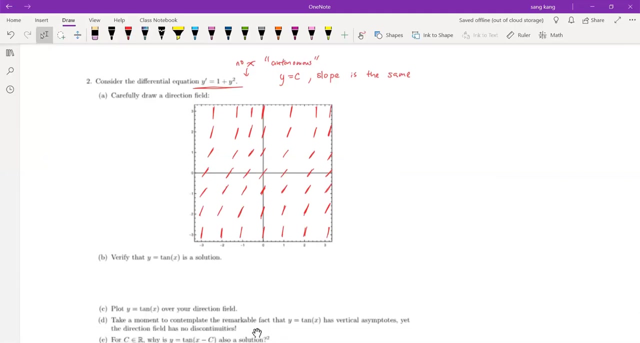 this is still 2, and then, or negative 2- it'll be a little bit steeper- and then negative 3, exaggerate it and basically draw a vertical line. second: okay, so that's my direction field, based on the differential equation. again, we can use the definition of autonomous to our advantage instead of looking at each 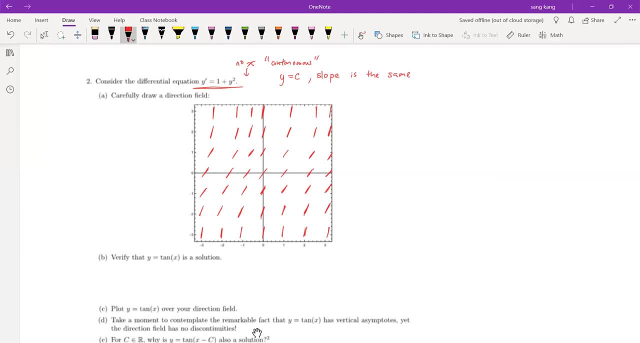 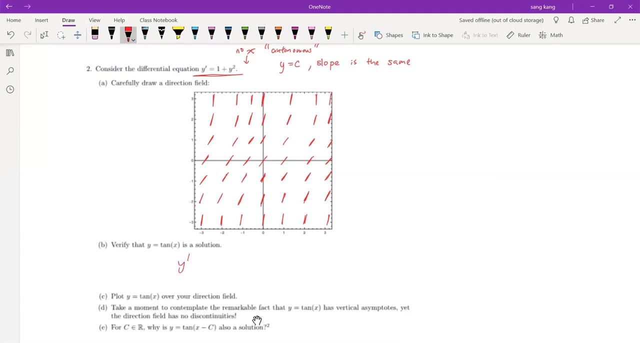 individual coordinate one by one. we know that for a constant, why the slope is the same along the horizontal, like that right. so now it says part B: verify that y equals tangent X is a solution. Y Prime is going to be 1 plus tangent squared X, so we're gonna replace this with secant. 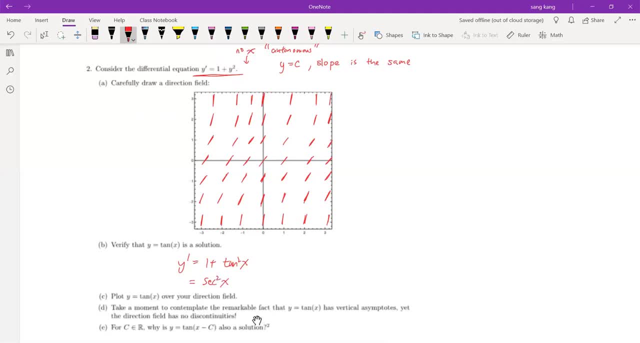 squared right, Trig identity. and now now we can. now we can plug y, prime back into our derivative number, and the psychologists you've probably j camped right to our differential equation here. So this would be: secant squared x equals 1 plus tangent squared x. therefore, secant squared x equals secant squared x. That's easier. 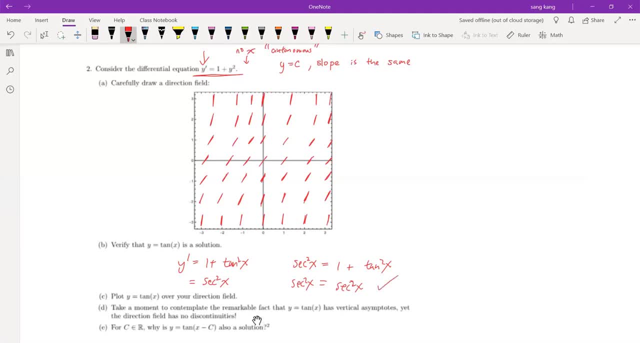 than the equation. Okay, so we verified that tangent x is a solution and part C is asking us the plot, our solution on this directional field. So if we start with .00, you would have something like this right, and you probably know what this graph is hinting at. This is: 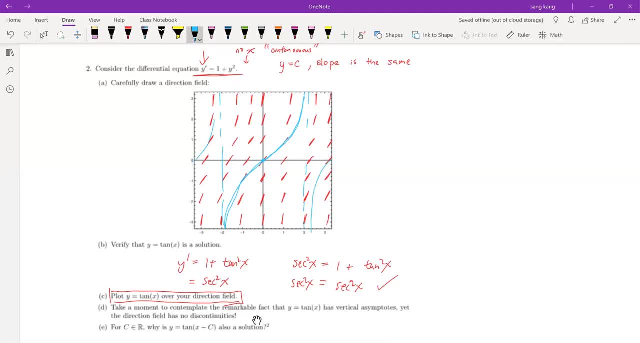 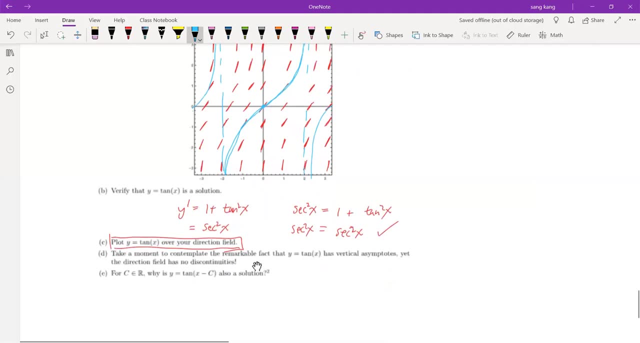 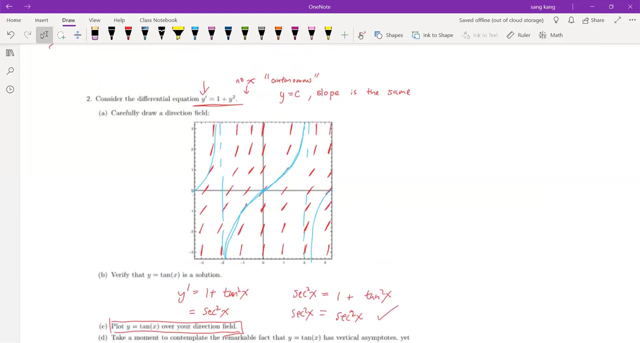 this is a. this is a, the graph of tangent right. Part D just says: take a moment to contemplate the remarkable fact that y equals tangent, x has vertical asymptotes, yet the direction field has no discontinuities. So no discontinuities, but we have. 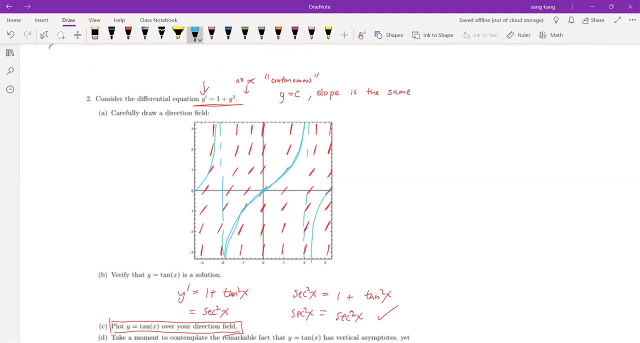 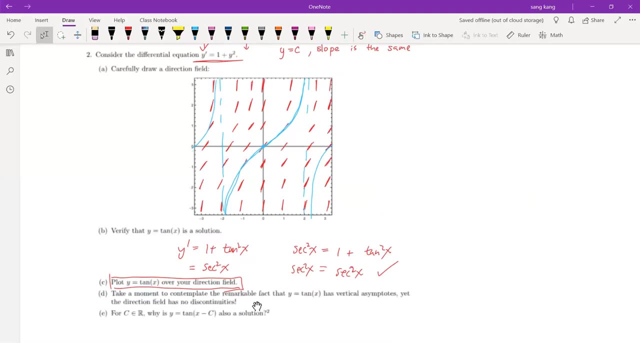 vertical asymptotes. but those are there for this particular case, particular case where particular initial condition. So now, if you look at part E, it says: for C, as a real number, y is y equal tan, x minus C, also a solution. Well, again, if we 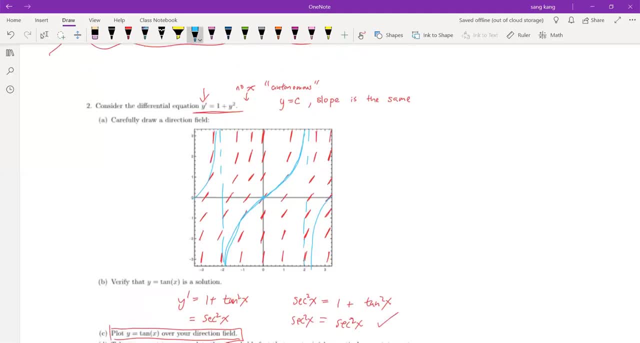 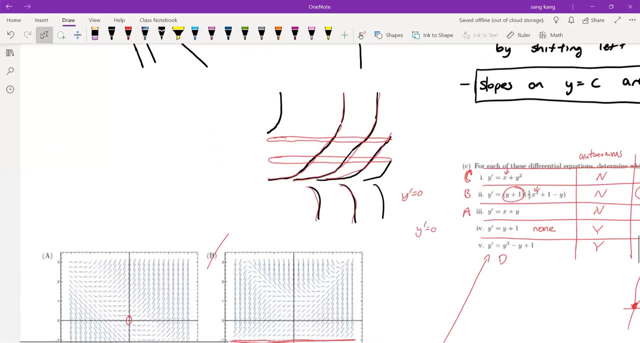 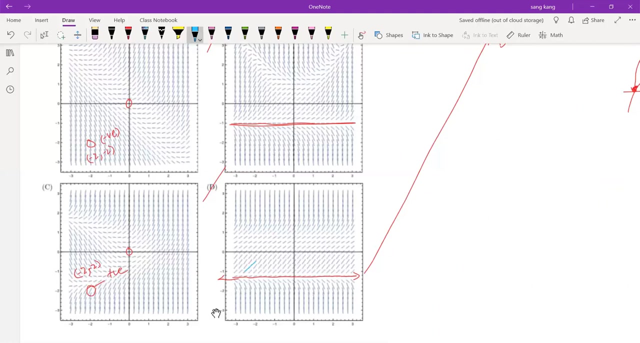 have an autonomous differential equation, we can shift it horizontally, left or right, and it'll still be a solution. So we saw that behavior. I kind of moved it, but remember that was this guy here, case D. So if you have a solution and we change the initial condition, all we're doing is shifting it. 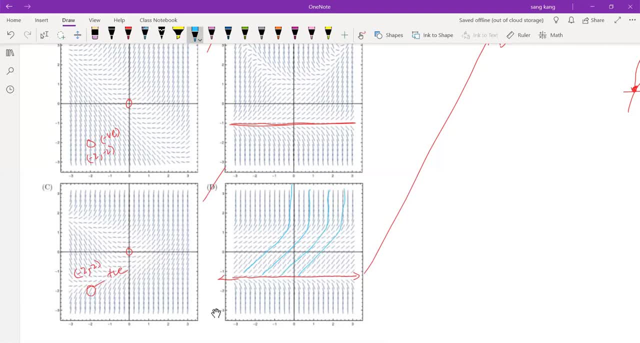 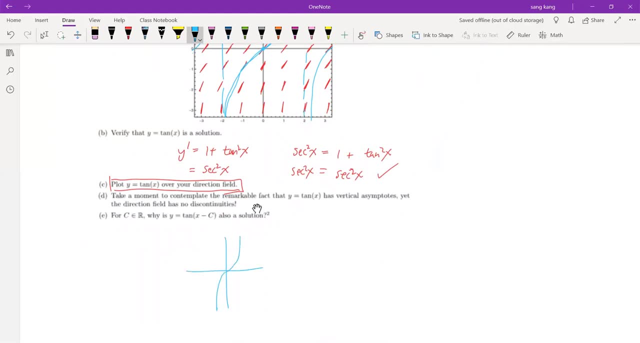 horizontally right. So that's the same idea here. if you have y equals tangent x minus C. if this is tangent, this is tangent, so this is my origin: 0.. X minus C is gonna shift it to the right by C, so this is C now right. So this is my new C. That's my new origin. Okay, so now. 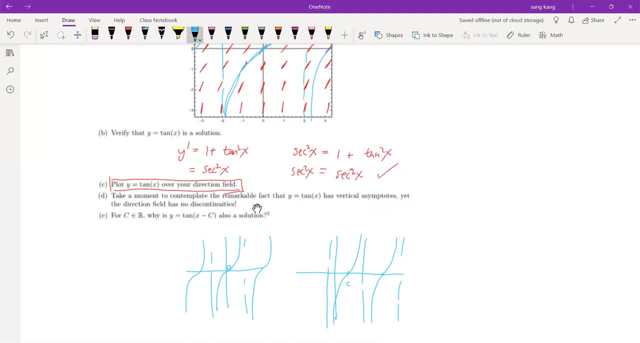 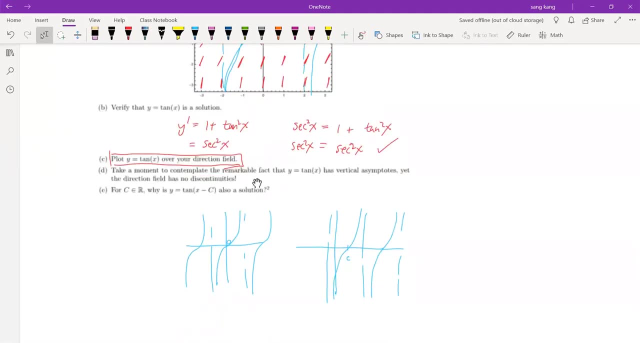 that is also a solution, and my asymptotes move. so that's basically what D is trying to point out. You know, we we have asymptotes but as a we're shifting it left or right, those will shift with it, right? Okay, let me screen capture this next one. Any questions on that one? 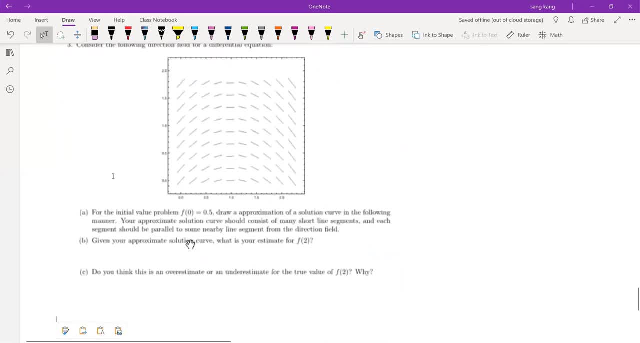 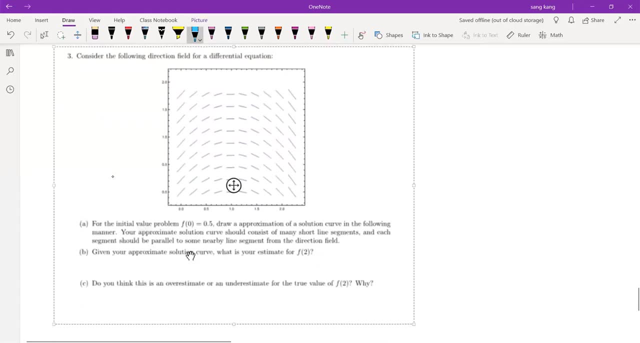 This sort of thing will take us a long way in finding those gak changes. Okay, for now we have this directional field. as for an initial value, if we start at, x equals 0, y equals 0.5, we're starting here, so this we're gonna. 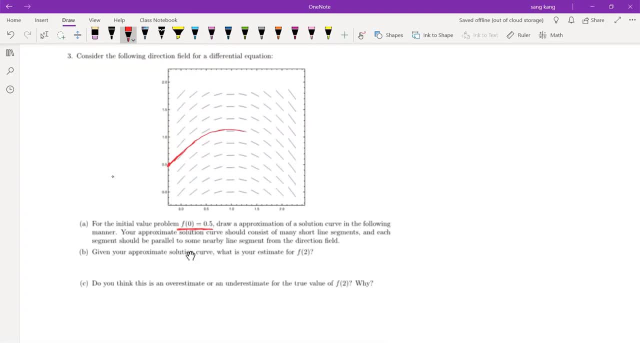 connect all these line segments right, so it'll look something like that. and now, given your approximate solution curve, what is your estimate for F at 2? so this is what we did, what I showed you earlier: we can use our solution curve to estimate values on our curve. so it: 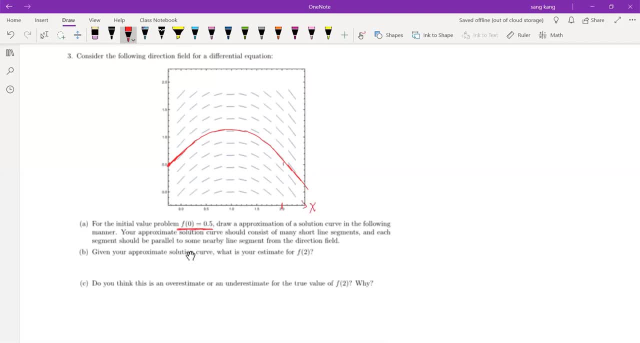 X equals 2, so we'll call this X- 2. you can see that we're somewhere here. we'll call that like 0.58 or something, 0.58. this is approximately equal to 0.58. I mean, this is completely based on your artistic ability, so 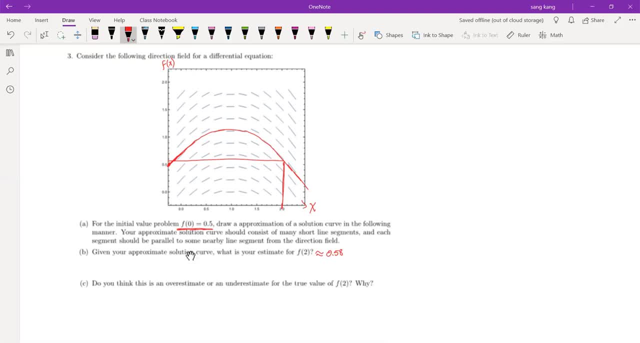 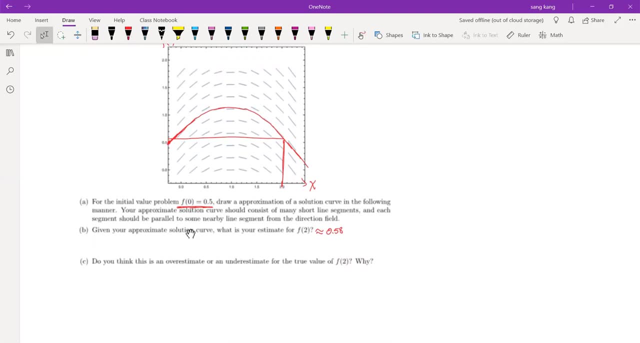 üzüg ναistyetzt Bayi. value of f, of 2 and y. so if you look at this solution- curve- remember these are all line segments, these tangent lines that I've connected to a smooth curve right. a good point. so we're going, action ist. 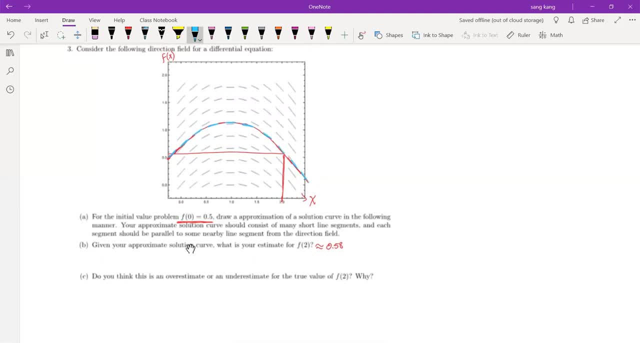 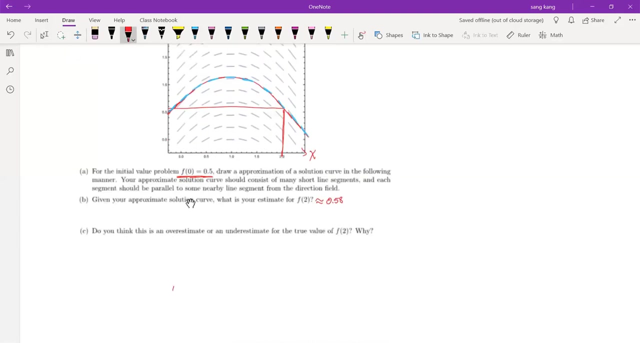 right. but really, when you think about it, these are a bunch of line segments that i just con, that i just joined in one smooth line, right, and also note that this solution- curve- is concave down. so if it's concave down and we have tangent lines everywhere, right, we have these tangent lines. 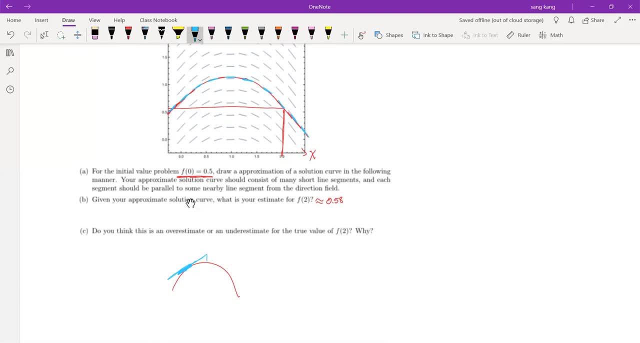 unless we land right on that point, we're going to have a slight error and because it's concave down, we're going to be slightly higher than that, than the actual value. so if this red line, with this red curve, was the actual solution and this tangent line, 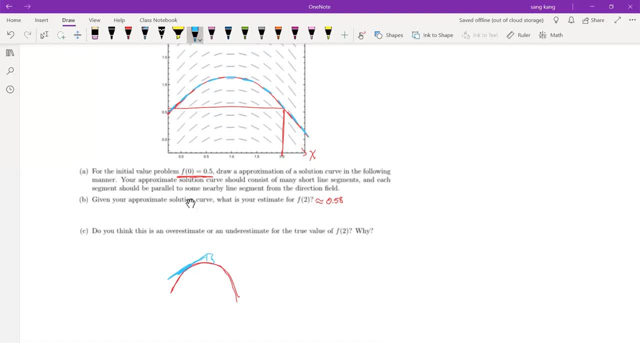 is our uh approximate solution right. so that's what's denoted in in blue in the in the solution uh, above we're going to have an over estimate because our solution curve is concave down. so this will be an overestimate, and the reason why is because of this, these facts. 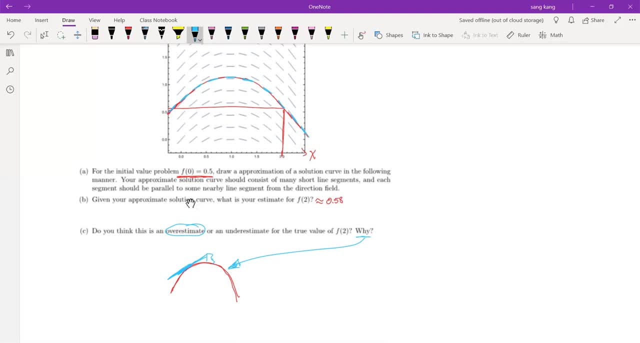 right, concave down, and we have tangent lines which slightly will overestimate. uh, if you, if you draw the tangent line to this curve, you can see that it's an overestimate. so obviously, conversely, if you had something concave up and you're looking at the tangent line, 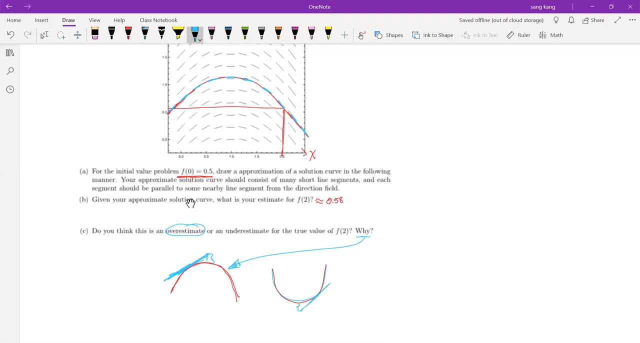 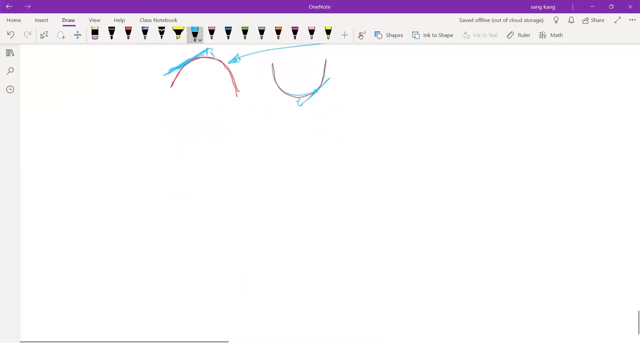 you would have an overestimate right, unless you landed right on that point. but we can safely say it's equal to or less than the actual thing. okay, so actually i didn't copy the last one, but it says: let's say so. they give you switch colors. 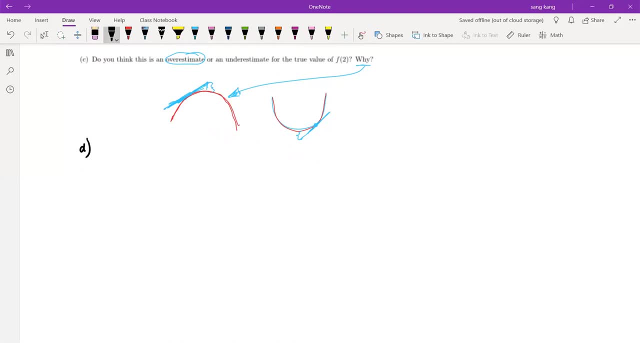 okay, part d. the differential equation for the solution curve of above is one minus x. so they give you that and they want you to find the exact, the exact value, find the exact value of f of two um. so all you have to do is find the integral of y. 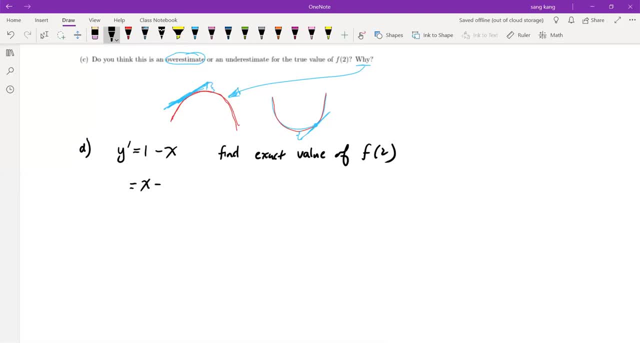 which is going to be x minus x squared over two plus c, and we saw that at f of zero this equaled a half. right? that was the initial condition that they gave us here, so we can solve for c. so from this, c will equal a half. and now, if we plug in,